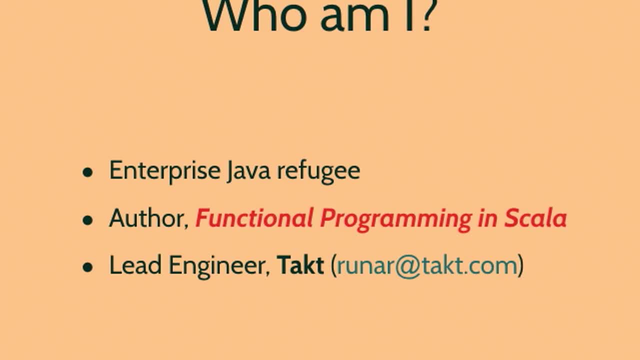 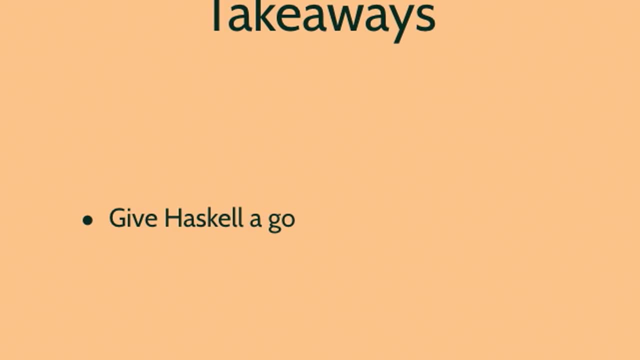 interested in working in Haskell all day. contact me at Renard at TACTcom. So in this talk I'm not going to teach you Haskell. My goal is really just to get you to be curious about Haskell and to just sort of give it a try. So the agenda is just one. 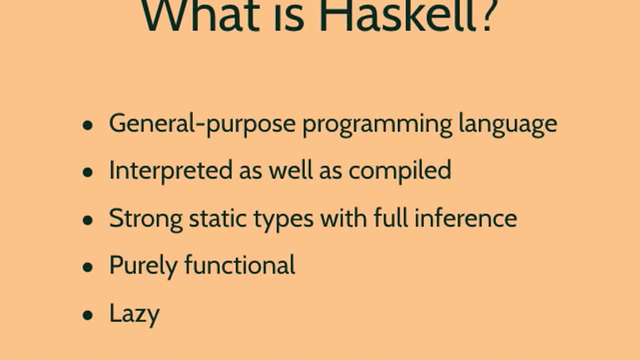 item. Please give Haskell a go, All right. so what is Haskell? Haskell is a programming language. It's a general purpose programming language. It could be used to make you know web servers and command line tools, games, enterprise software. 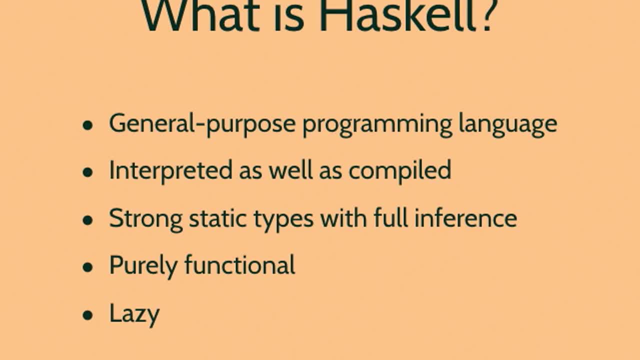 as well as you know other programming languages. It's a popular language to implement other programming languages in, So the Haskell language itself is separate from the implementations of Haskell. The most popular one is the glorious Haskell compiler, which compiles Haskell to native code as well. 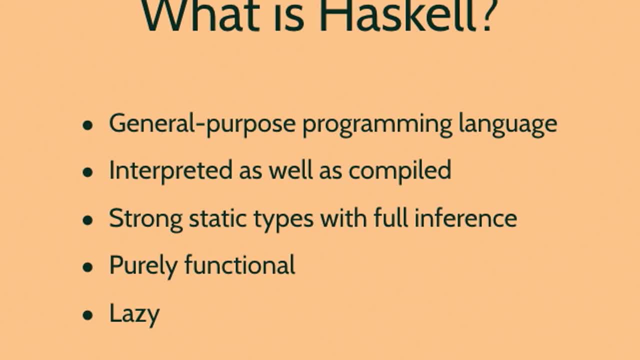 as C and LLVM compiles it to JavaScript or Java bytecode. So there are lots of different back ends for GSC but the most commonly used one is the native compiler Or you can- you know you can- compile to GHC's own bytecode. 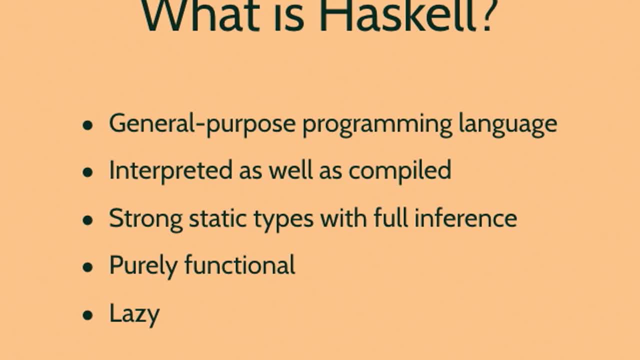 Which then gets interpreted by the GHC runtime. So Haskell itself is not opinionated about whether it's compiled or interpreted Well. Haskell has strong static types and it has full type inference. So we you know we tend to talk about types a lot in Haskell, but Haskell is actually able to infer most. 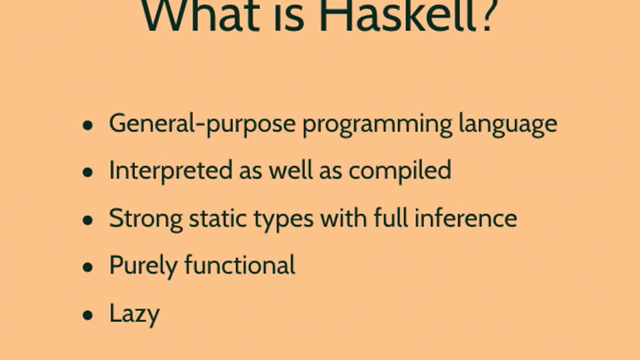 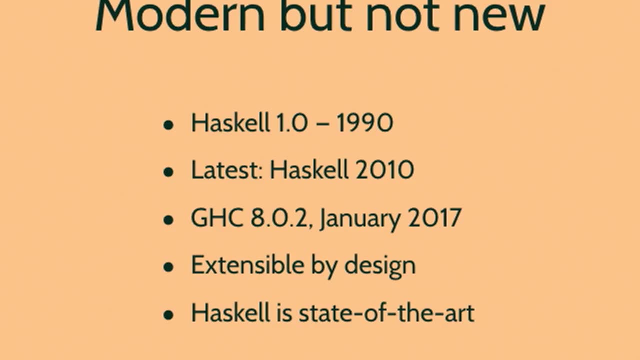 of the types. for us, Haskell is also purely functional And it is a lazy language And I'll go into what that means here in a bit. So Haskell stands at the end of decades of programming language research. It started out as Haskell 1.0 in the year 1990.. So it's sort of venerable. The latest Haskell language. 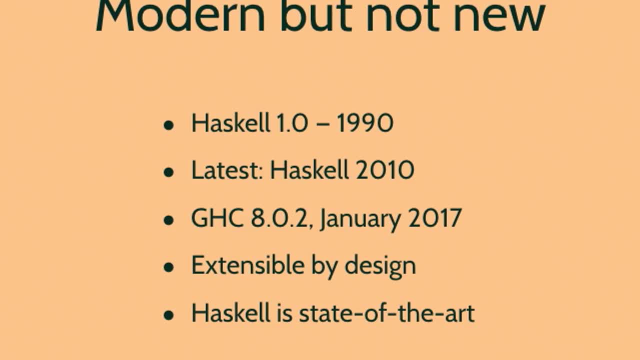 reference is Haskell 2010.. And the most modern sort of up-to-date implementation of a Haskell compiler. Haskell is a glorious Glasgow Haskell compiler which is in version 8. And 8.02 came out in January of 2017.. And it's in active development. They're constantly adding new things And 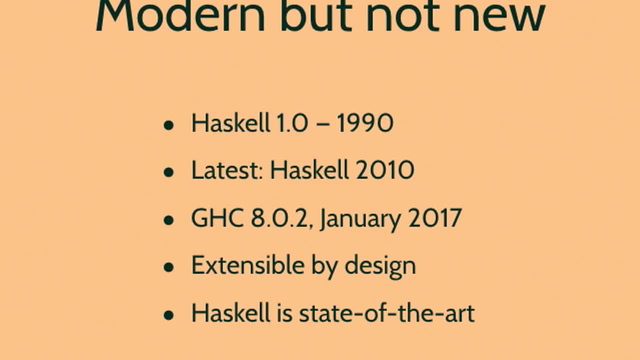 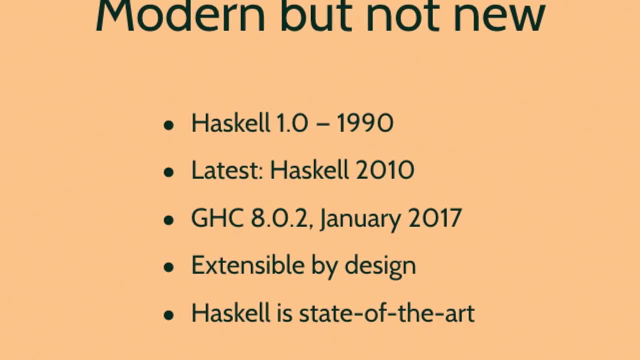 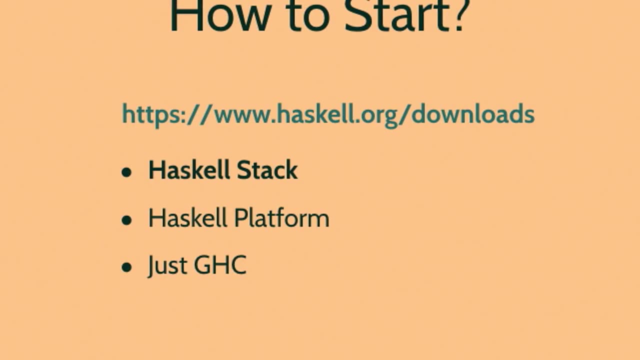 But it's a lot. new thing comes out in programming, language research, like dependent types or linear types or other things like that. They find implementations in Haskell pretty quickly, So those things become available in Haskell quite quickly, All right. So how to start in Haskell? Well, you go to Haskellorg and you can download. 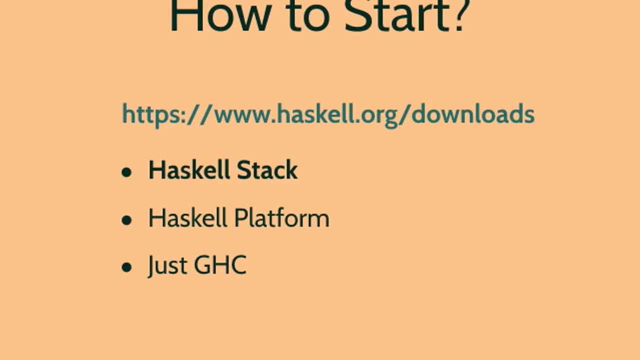 either the Haskell platform or you can just download the Haskell compiler, But the recommended method for beginners is to download the Haskell Stack, which will allow you to get up and running really quickly. It comes with a bunch of libraries that all work together and is 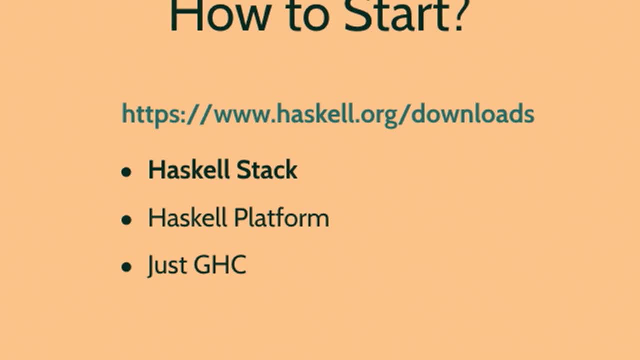 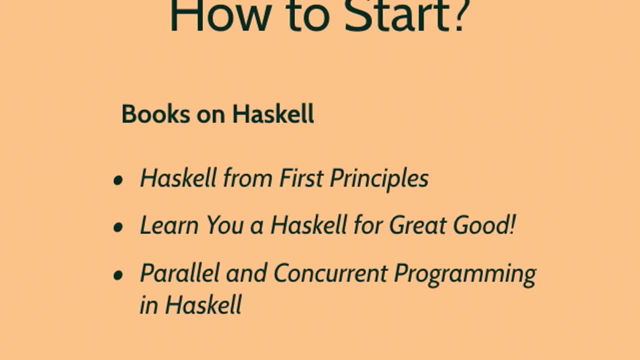 sort of opinionated about how you structure your Haskell project and things like that. So Haskell Stack great for beginners. There are lots of books on Haskell. Some recent ones are Haskell from First Principles by Chris Allen and Julie Mornucchi. That one. 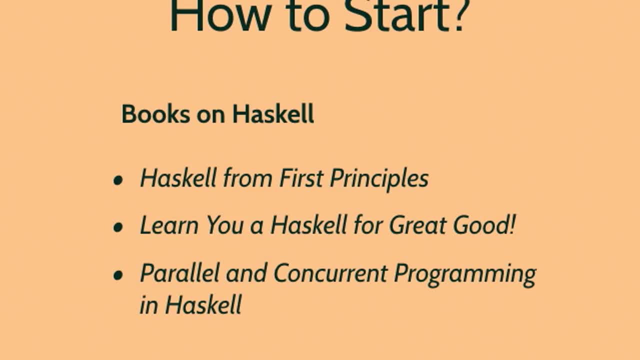 is really great and it's pretty new and very up to date. with regard to Haskell, There's a sort of a little bit out of date one called Learn You a Haskell for Great Good, which is super fun. It's an awesome book to go through. And then there's a recent one which is a little 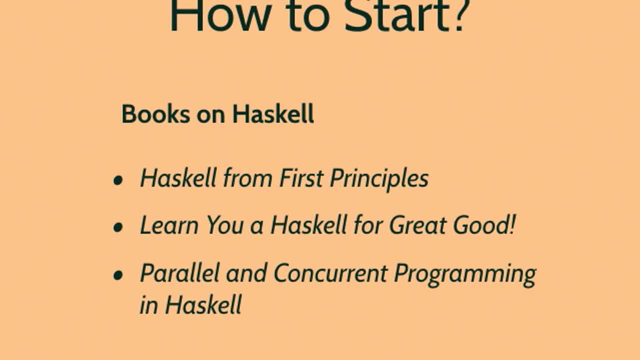 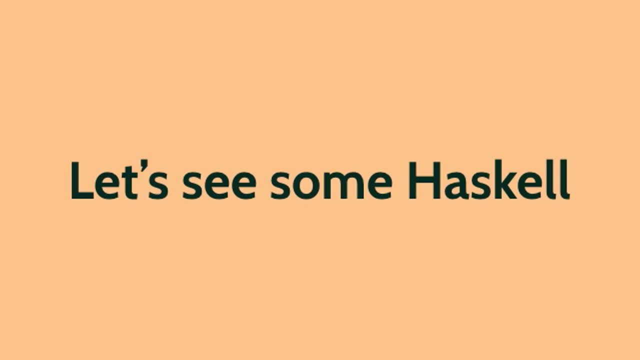 more advanced, which is called Parallel and Concurrent Programming in Haskell. I believe that one is great. This is by Simon Marlow. Okay, so let's see some Haskell, right? Yeah, let's go see some Haskell. Okay, so if we 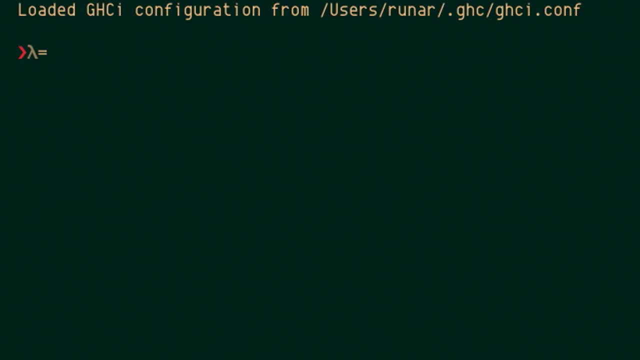 start up GHCI from a terminal. we get the Haskell read eval print loop with the Haskell interpreter. Okay, Oh, I'm really sad that this is cutting off the top of my slides. Yeah, Can we fix that somehow, I wonder? Yeah, I'm missing a whole line at the top here. 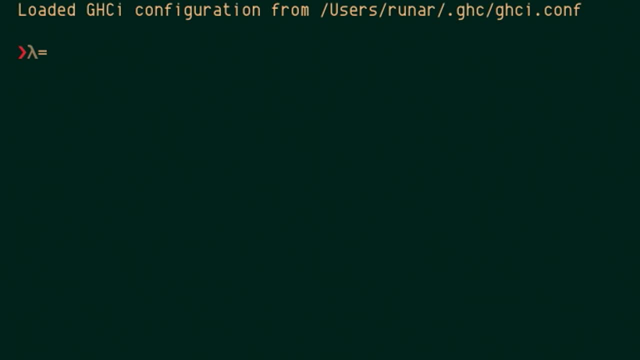 It's actually slides, isn't it? Yeah, it's actually slides. God, I can start pressing buttons if you like. No, that's all right. I mean, maybe it's the angle of that, What do you think? No, it's actually cutting it off. 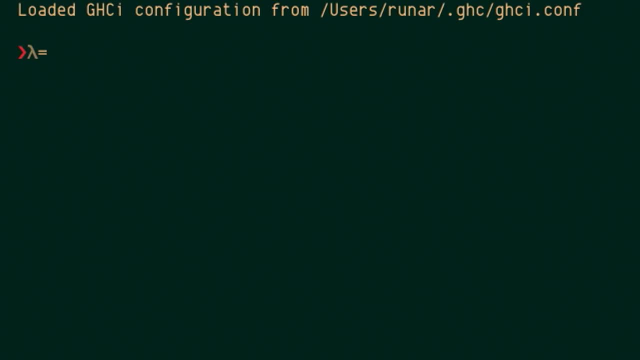 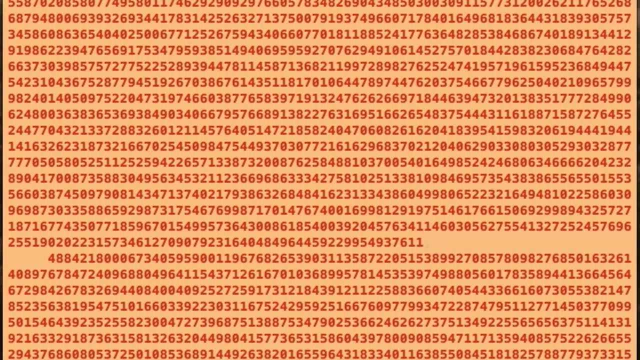 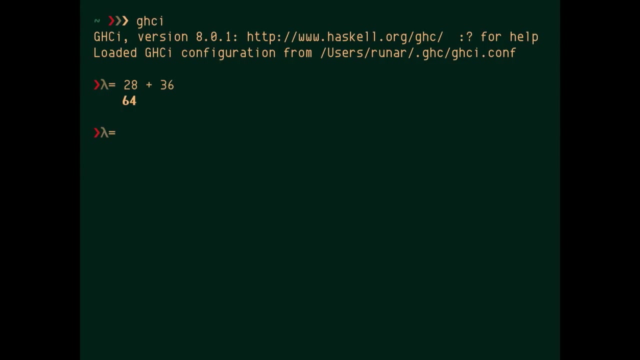 Okay, well, maybe I can try to switch into that, Because it would be great if I could actually show my slides. Sorry about the slight delay. All right, so if we fire GHCI from a terminal, we can just start typing in Haskell expressions and they will be compiled to Haskellbycode. 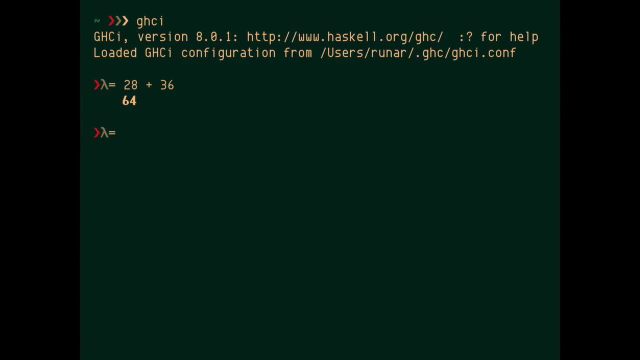 and they'll be interpreted. I can type in arithmetic expressions like this and I can apply function to arguments. You'll notice that Haskell is very sort of syntax light. It's a very quiet language syntactically. The syntax for function application is just space. There are no parentheses around arguments. 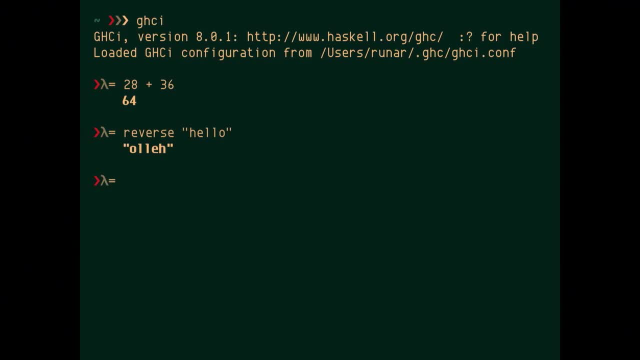 Here I'm passing the string hello to the reverse function. I'm getting the reverse. I want to pass two arguments to a function. I just separate them. There we go it then by spaces. So here I'm checking if p is an element of the string xellophone. 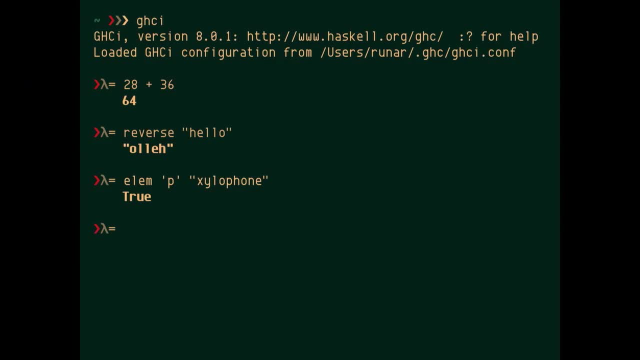 which it is. so I get true. So again, Haskell, very sort of quiet, But we can use parentheses to disambiguate. So here I'm passing the sort of the list 4, 1, 2 to reverse rather than. 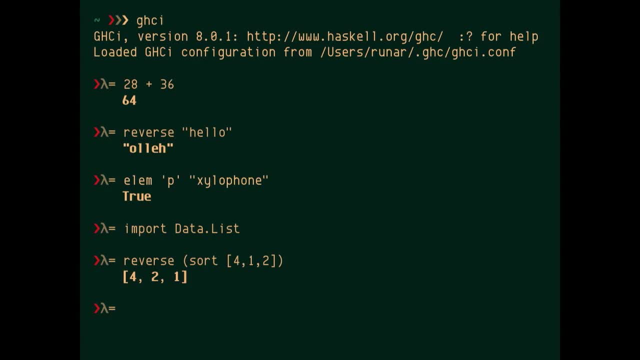 passing the sort function and the list as arguments to reverse. So first I want to sort and then I want to pass that to reverse. So, speaking of which, Haskell is a functional language and so functions are first class values, And so here I'm creating a function. 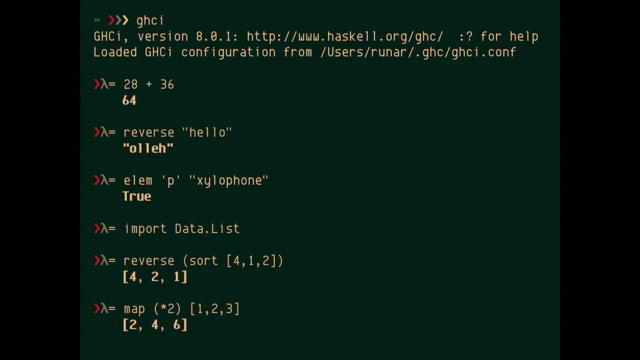 in line that multiplies its argument by 2.. And so I just put parentheses around that and just say times 2.. And if I pass that to the map function together with the list, it will apply my function to every element in that list. Yes, 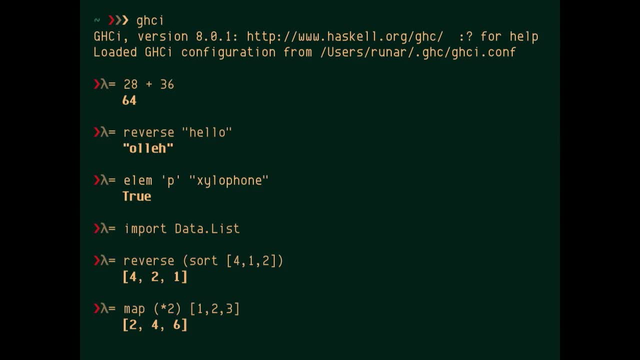 Can you make the parentheses that disambiguate? Yes, otherwise it will infer that as map times 2, right Got it, Yeah, So I need the parentheses around times 2 to say that this is a function that takes an additional argument. This, sorry. 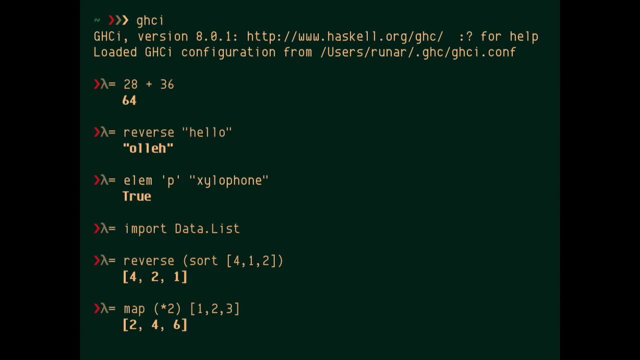 Oh, if I said, map parentheses, 1 times 2?? Yeah, Oh, that would not work. That's a type error, Because 1 times 2 is a number, but times 2 is a function that expects another right. So it's really. 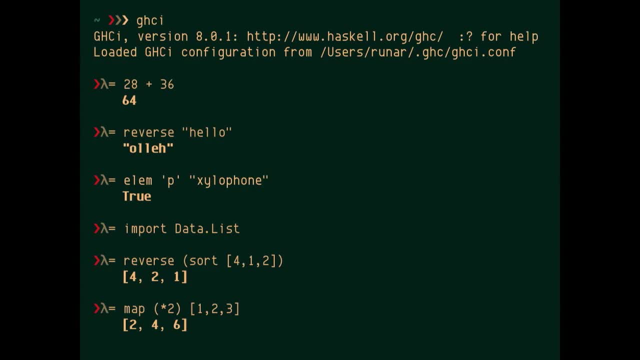 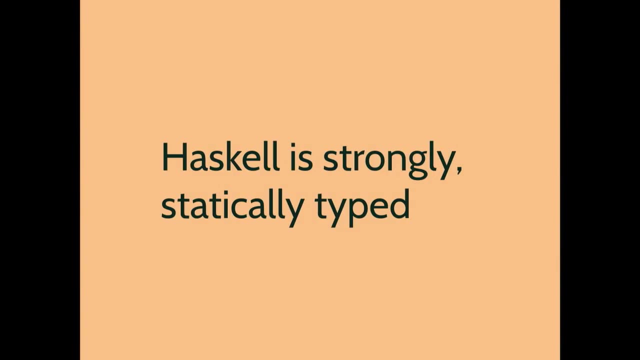 Yeah, the first argument: to map should be a function, So speaking of which Haskell is strongly statically typed, So we're able to type in all of these expressions without ever mentioning any types, right? But and that's because Haskell actually infers the 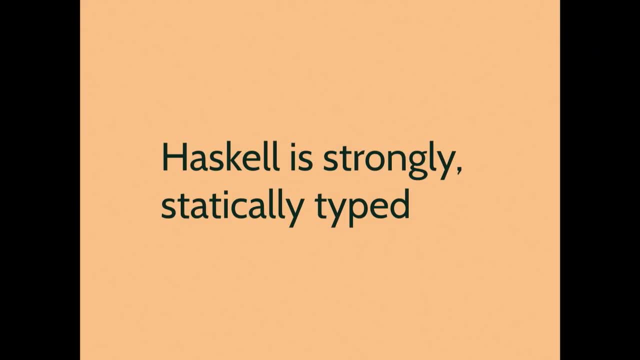 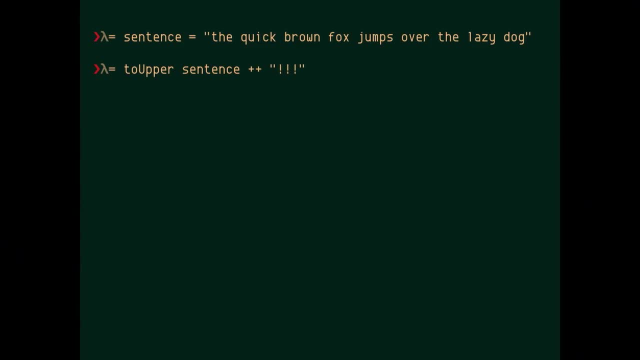 types for us. But Haskell is strongly and statically typed And that's really great because you know, types alert us to mistakes super quickly, For instance here. you know I might want to take this sentence here and it's not really. 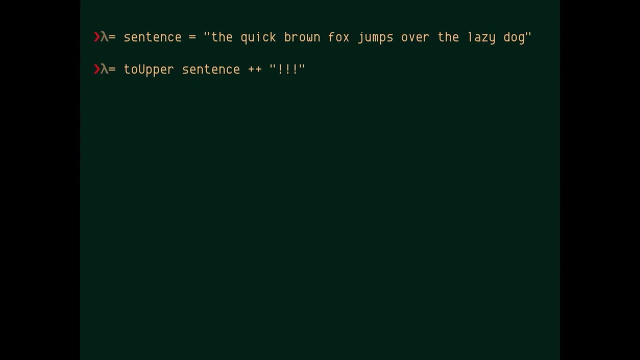 loud enough for me. So I want to like turn it to uppercase and like append three exclamation marks and maybe like a damn it on the end, And so you know I might think like okay. 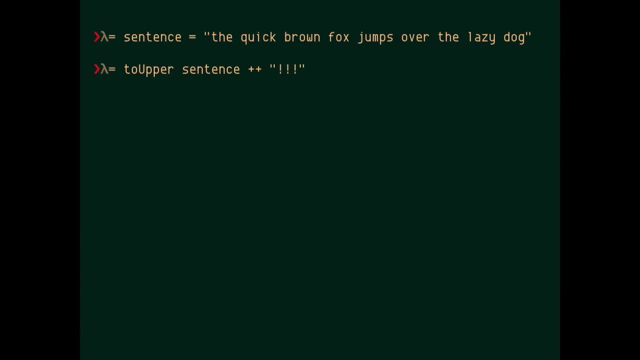 well, I'm just going to two-upper that sentence and then append three exclamation marks. Okay, And 그러면 Haskell comes back and says: no, You cannot do this because, well, I expected to see characters, but I actually saw lists of characters. 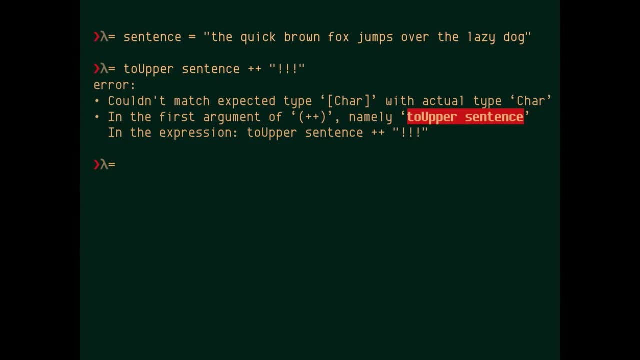 And it's telling me where the error is – the type error – comes in two-upper of sentence. So then I can actually ask Haskell: well, what is the type of two-upper, What's actually wrong here? And Haskell comes back and says, well, two-upper takes a character. 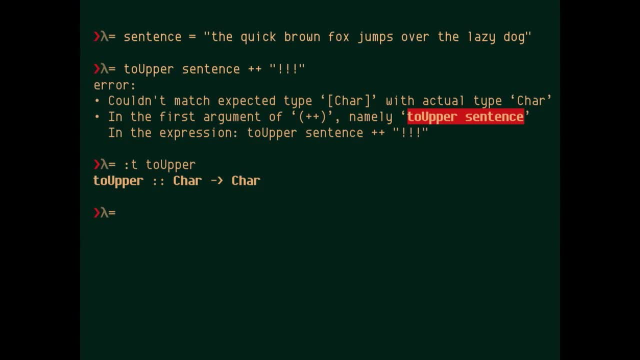 and turns it into a character. the colon colon reads: has type, so toUpper has type car to car. so it's a function that takes a character and returns a character, So it actually operates on individual characters. So I have a function that can turn such a function into a function that operates on 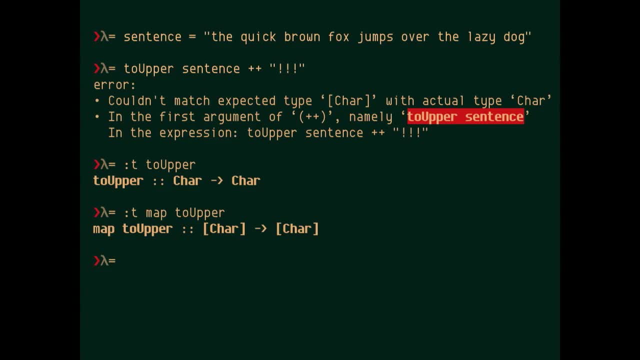 lists. So if I say map toUpper then that becomes a new function that applies toUpper to every element of a list, and in Haskell strings are actually just lists of characters, And so now map toUpper enables me to apply toUpper to every character in the sentence. 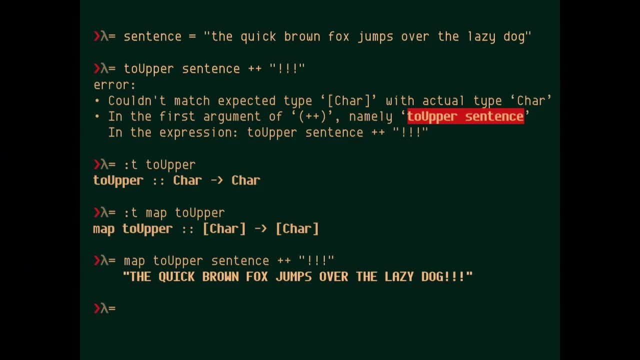 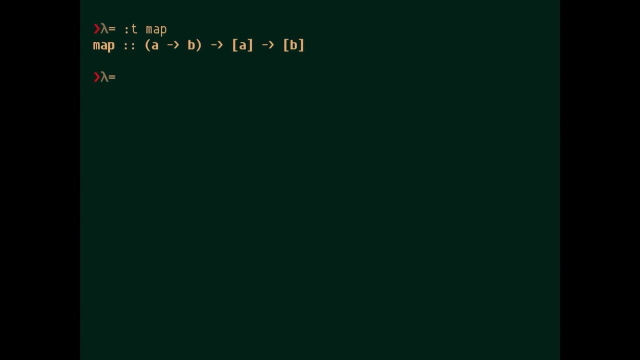 and now the quick brown fox really does jump over the lazy dog. Cool, so static typing for the win. It's really easy to make mistakes like this, and Haskell catches them super early. So now if we ask for the type of the map, 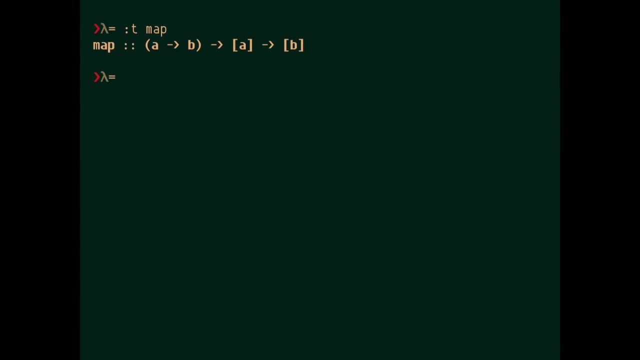 function. Haskell comes back and says: well, map has the type like this: It takes a function as its first argument, from A to B As its second argument, it takes a list and it returns a list. So it takes a list of A and it returns a list of B. given a function from A to B, 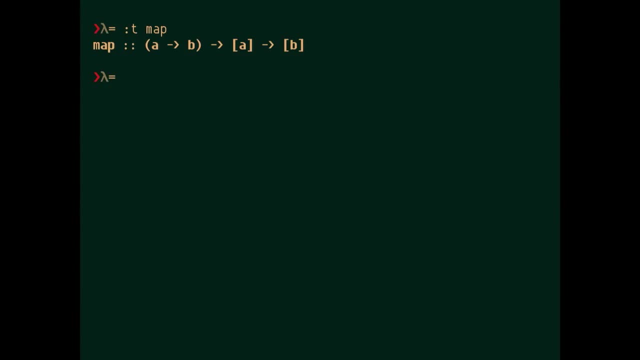 Another way of reading that is that map turns a function from A to B into a function from list of A to list of B. So in Haskell actually every function just takes one argument. And the way that Haskell implements functions that take two arguments is that the function will just return another function that takes. 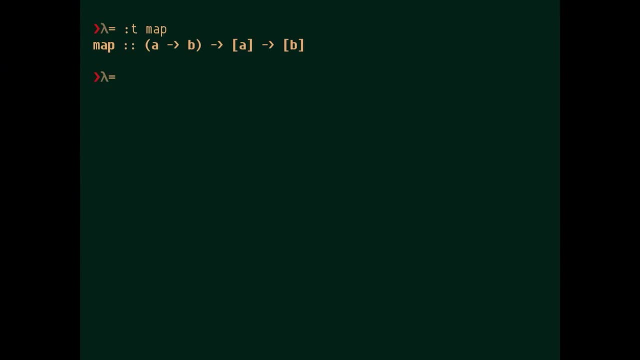 the next argument. So map is actually a function that takes one argument and it returns a function that takes the list as the next argument. So every function in Haskell is curried Okay. so what are these A B things? These are actually type variables, So it's not a. 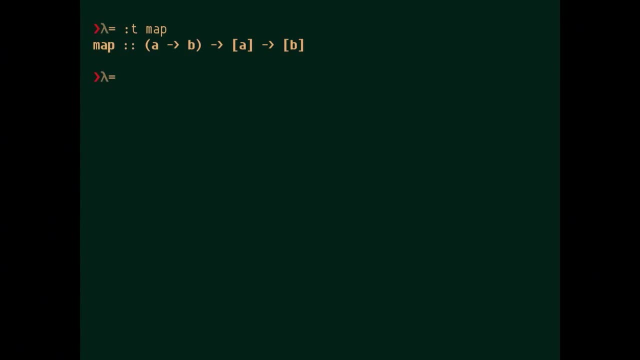 script. it's actually a display like a map. So this is a graph of a map. You can actually do the math with a graph like this and get the same kind of result. So in Hackensack you can actually look up this graph on a computer, but you can't actually get the exact. 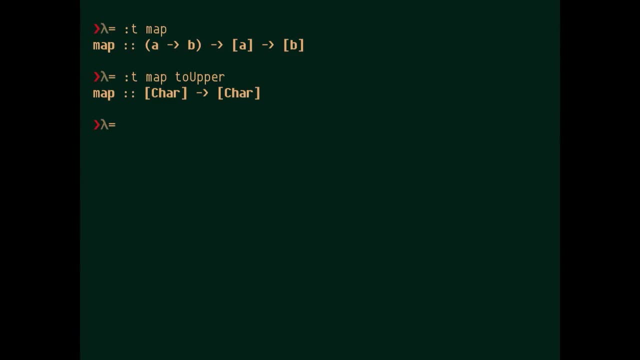 result that's coming out of it, And so we asked it: okay, how many types of a-a- and I'm going to pick a few types that are actually polymorphic- You can actually specify what these types are, That's so. they are generics, essentially. 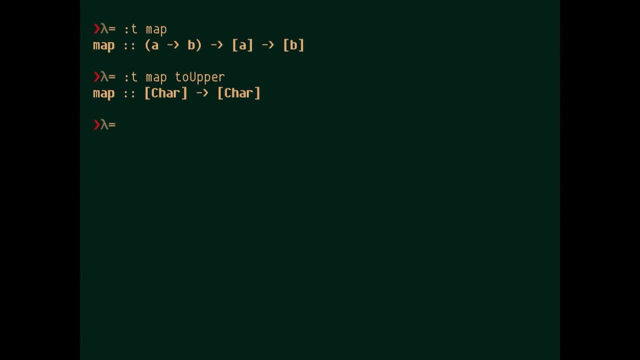 So so the type of map is actually polymorphic And we'll get into what that means here. and B to be char. Now I've assigned these type variables to be the char. type Map will actually work for any two types, A and B, With map to upper. actually I'm setting them. 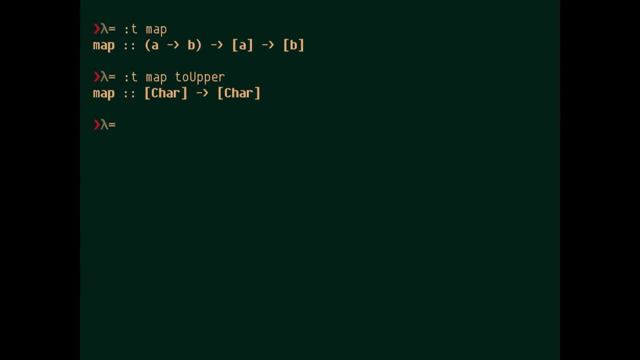 both to be. char Map is polymorphic. It's not just functions that have polymorphic types in Haskell, but values can be polymorphic as well. Functions are values, but values other than functions can be polymorphic. For example, the empty list. if we ask what is the type of the empty. 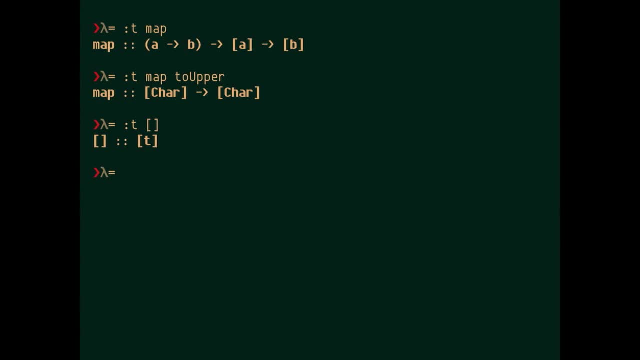 list. Haskell comes back and says: well, the empty list has type list of T for all types T. It doesn't matter which type we pick as the element type of the list, It has no elements. so it's the list of T for all types T. In fact, the empty list is the only list that 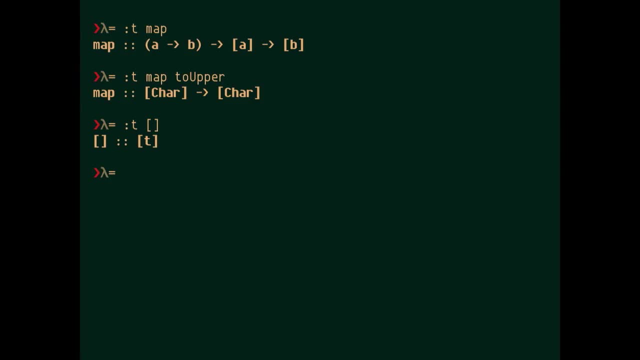 has this polymorphic type. If we have a value of this type, we know that it must be empty. That's actually kind of cool, because sometimes a type tells us everything we need to know In Haskell. often the types will guide you towards an implementation, or will guide you towards a correct implementation. 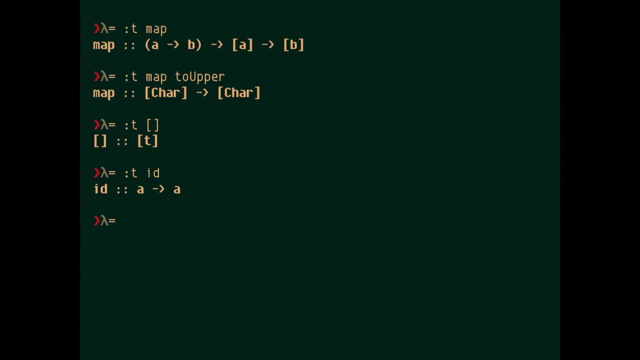 of your functions. For instance, if I ask, well, what is the type of the identity function? The identity function takes an A for some type A and returns an A for some type of function. It returns an A for the same type A. This type actually tells us what the implementation. 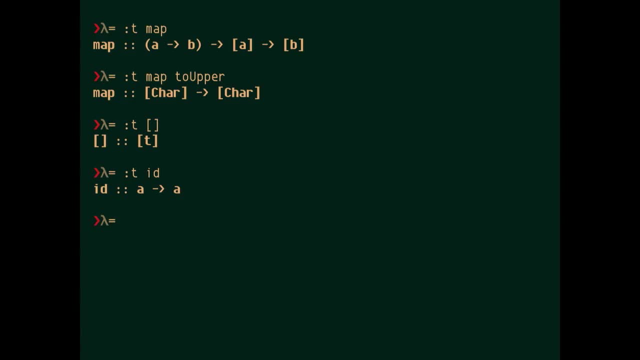 of id is It must return its argument, because that's the only way it can get an A to return from that argument, because it has no way of knowing what is the type of the thing that you're going to pass in. This type completely determines this implementation. Here's another. 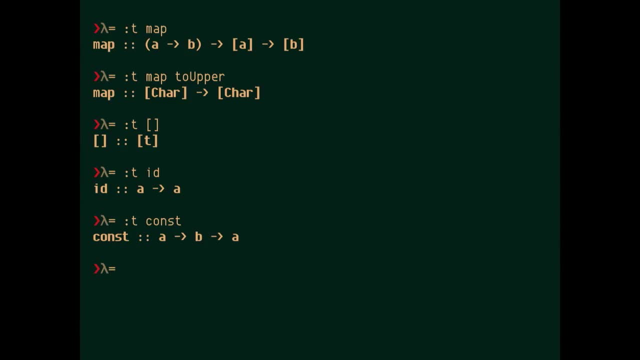 one. that also It does. that You can see if you can guess what this does. Const takes an A and a B and returns an A. It must return its first argument. It takes two arguments and it has to return the first one. That's the only thing this function could do. 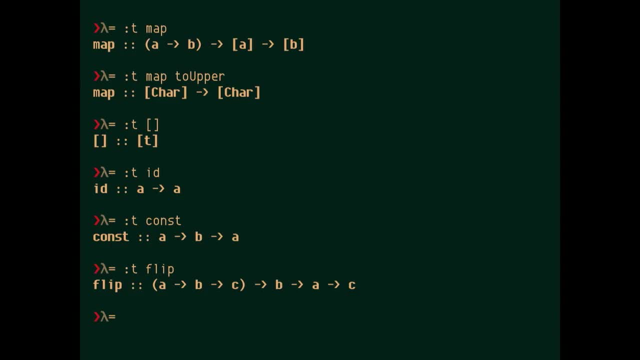 More complicated one here. Flip takes a function that takes two arguments and it returns another function that takes two arguments. The function that it takes takes an A and a B and returns a C. The function it returns takes a B and an A and returns a C. 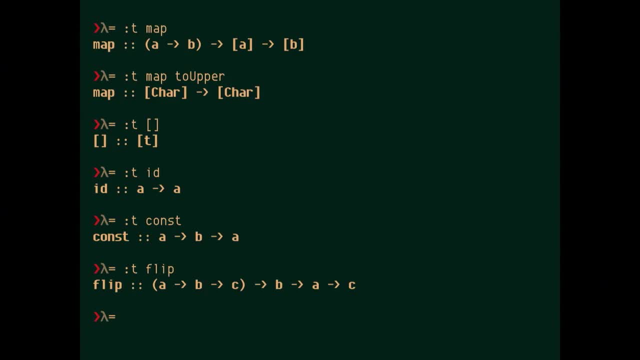 It flips the arguments. A fun exercise is: what is the type of flip-flip? It will move that B over to the beginning. Flip-flip will be a function that takes a B and a function from an A and a B to a C. 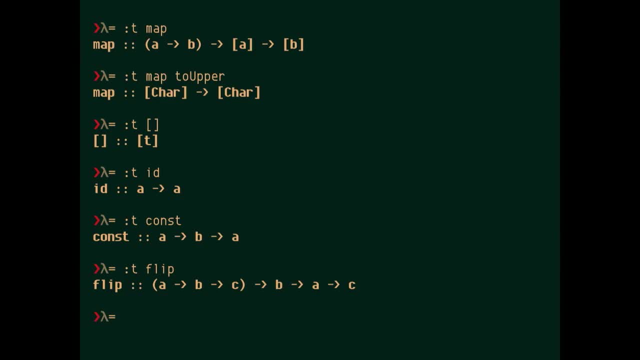 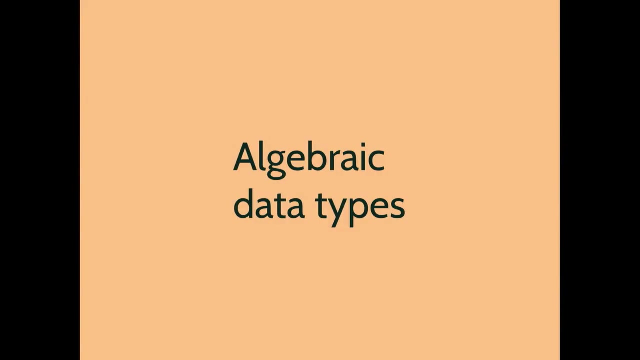 and then applies the B and the A to the function that it got. Anyway, Haskell allows us to do this sort of arithmetic with functions. essentially, Functions are very, very much first-class values. Haskell also has algebraic data types. We can specify our own types. They're algebraic. 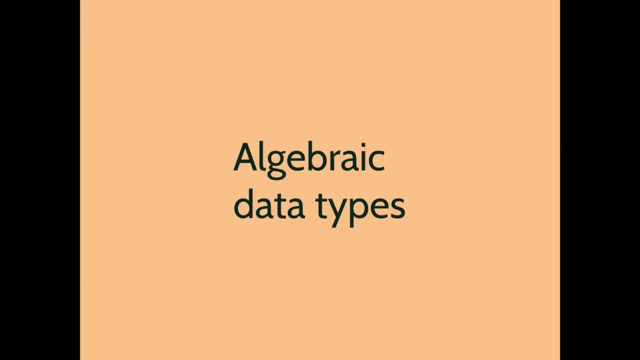 in the sense that they are composed of. They have an algebra and the algebra is that they are composed of ands and ors. It's sort of like a Boolean algebra. No, They're similar, but lowercase. I'll put this in. That's the reason. 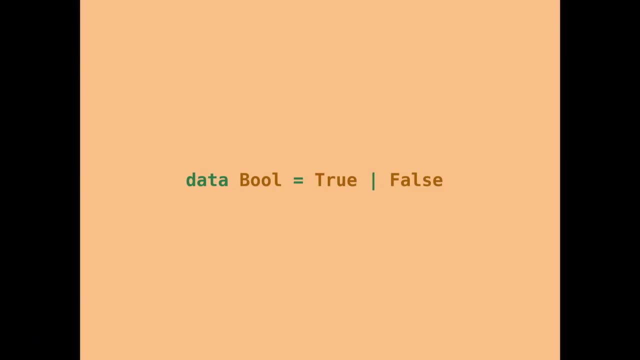 So this iscurrently hintenised? Yeah, that's what I meant: Off canvas or fallow canvas. I'm trying to identify how we're writing these, For example, if this weirdEyes item, I'm not sure the answer to this one. 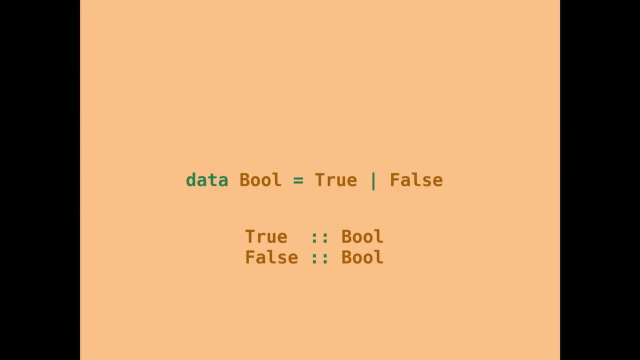 I mean, I got almost 50% of it. Ok, So we'll say: one dot everywhere. two data constructors are the only two ways that you can construct a bool. There'll be two values in scope- true and false, and they're both of type bool. That was one or the other. 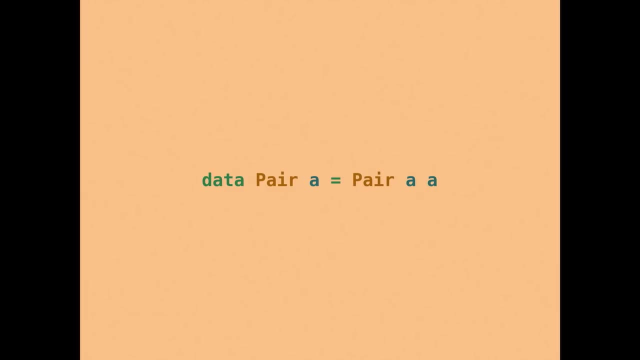 You can also do and pairs of things. Here is a simple pair data type. Pair of A has a single way of being constructed. It's a pair that takes two. As What that does is, it creates a single constructor called pair. It takes an A and an A and it constructs the. 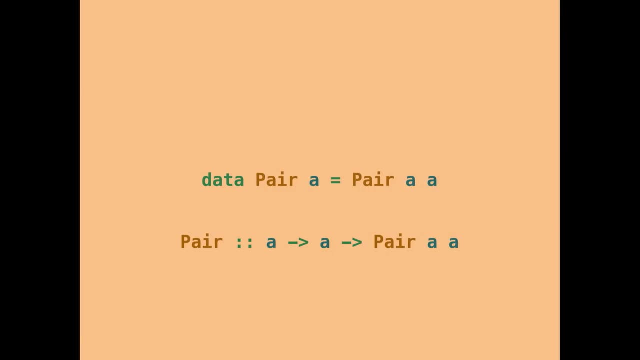 pair of A and A. It can be a little bit confusing to beginners that the type and the constructor have the same name. but that's sort of similar to what you would see in languages like Java. In practice we don't actually confuse types and constructors because one is at the 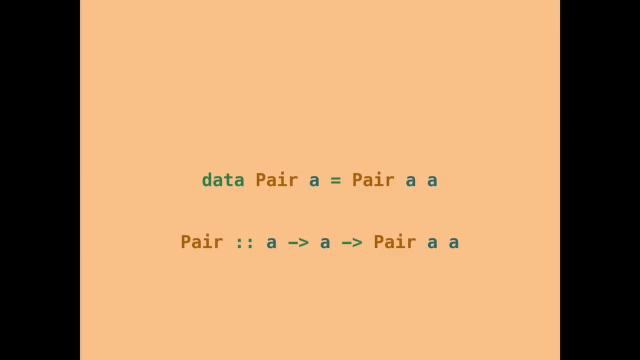 type level and the other one is at the value level. We normally don't talk about them in the same context. We can also combine and and or or products and sums by just nesting things. Here is a simple binary tree. It's either a leaf which contains an A or it's a node that contains 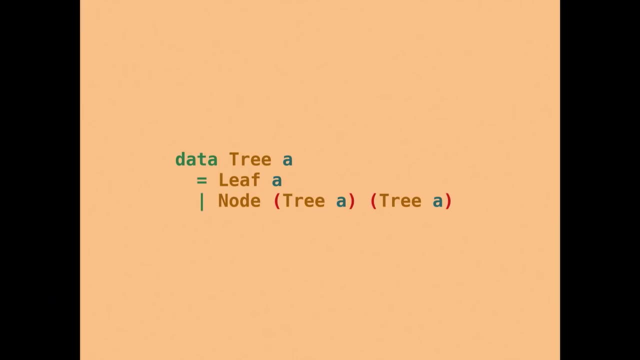 two trees. It's a recursive data type. This A thing is a type variable. This is a generic type. It's not specified what the type is of the values that we put in the leaf. It could be anything. Tree of int is an example of a concrete type. 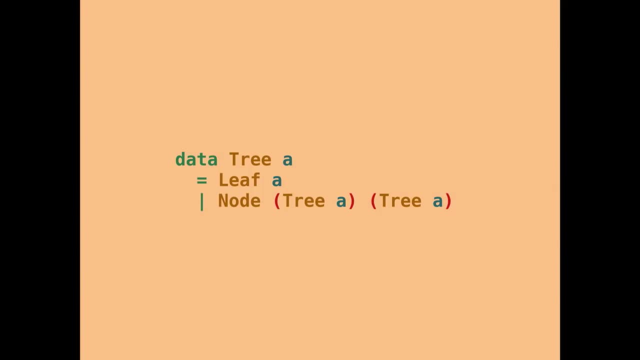 Is node inside the tree. Sorry, I didn't catch. that Is node. what? Is this a one-liner or does node have to get declared on the previous line? Oh yeah, This can all be put on single line. This is just formatting for sort of niceness. 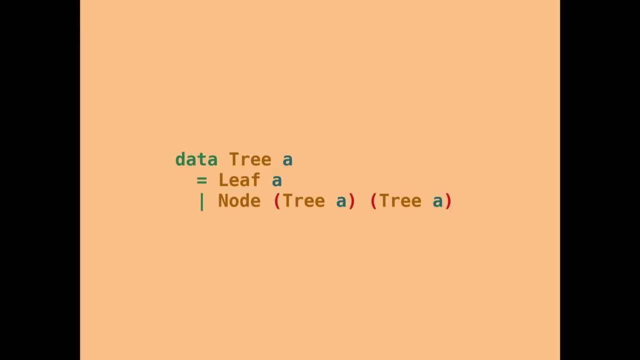 It's defined in this line that we see there. So you define the tree data type, which two value constructs are one line and two tree and one number. It's another form of a linear node. Right, Yeah, Yeah, Yeah, Yes, okay, yeah, so this is defining node. 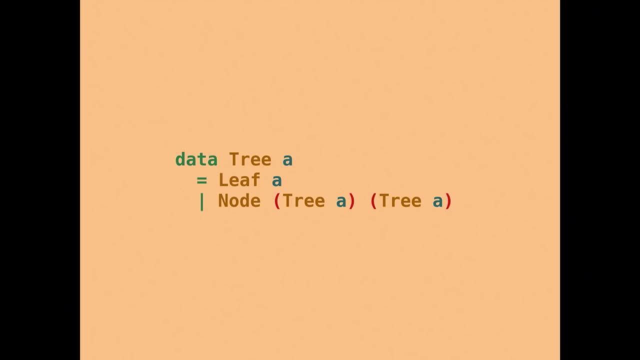 So this is saying the definition of node is that it's a constructor of tree and it takes two trees as arguments. right, Cool, so that's algebraic data types. Another really cool feature of Haskell is that it has type classes and type classes. 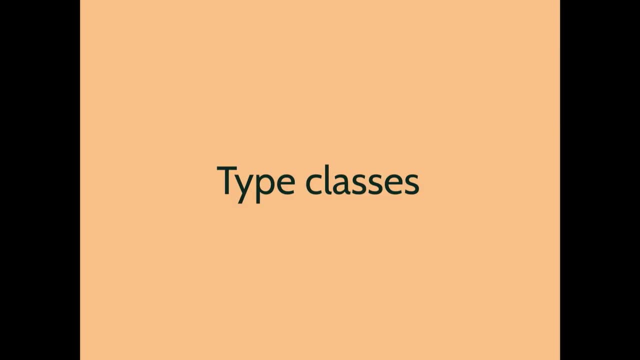 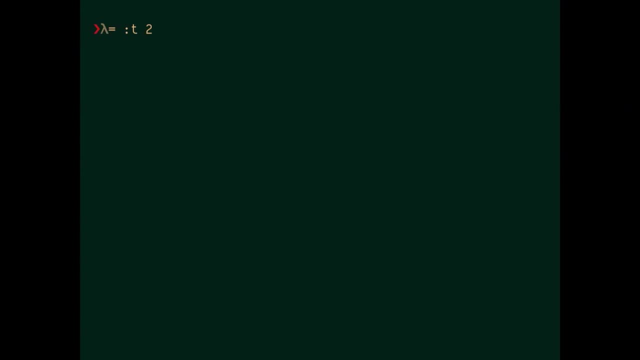 are sort of unlike anything you might see in other languages. I believe that this actually originates in Haskell. So if we ask what is the type of two, Haskell will come back and say: well, it's not a concrete type like integer or something. 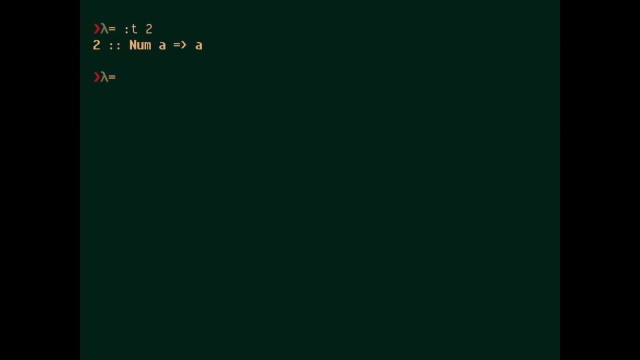 It says it's of type A, but this reads: two has type A, given that A is a number type. So, given that A is of class num, two is of any such type. So two can play the role of a float or an integer or whatever implements the numeric. 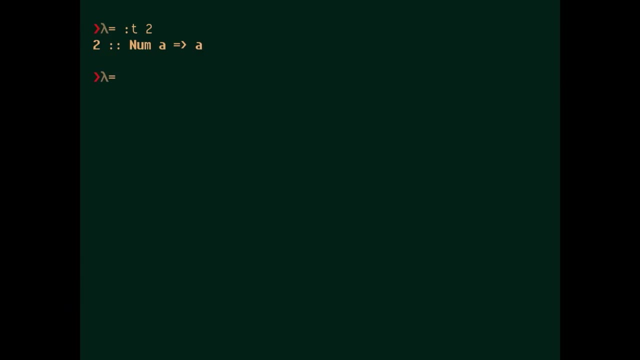 interface. So num here is called a class or a type class, and it's not really similar to OO classes. It's more like OO interfaces. but it's actually not like that either. The proper way to think about this is that it's a classification of types. 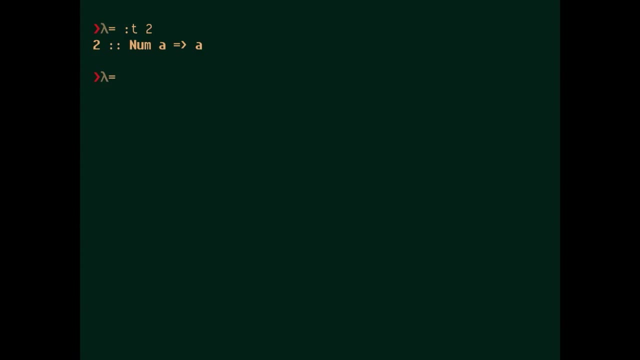 So there's a class of types, There's a grouping of types, all of which are numbers or are numeric, So they have to implement this num interface. Another example of this is the type of equality. It says that the type of equality is. it takes two As and returns a bool, but A has to be. 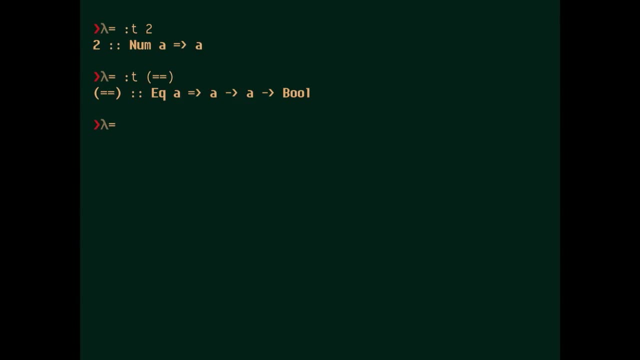 of class eek. It has to be an instance of this class. So somebody has to somewhere specify what is the definition of equality for your type before you can actually compare them for equality. And lots of those are built into the standard language, Like, for instance: we can compare two lists for equality and we'll get true. 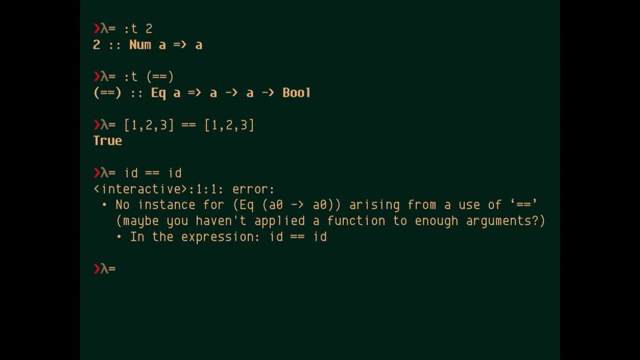 But if we try to compare two functions for equality, we actually get a type error And Haskell will tell us: there is no evidence or there's no instance for eek. There's no evidence that I'm able to compare these two functions for equality. 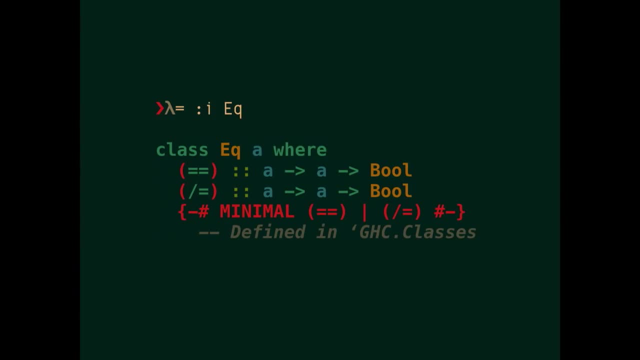 And we can ask Haskell for more information about the interface provided by a type class. In GHCI, we can say colon I, which is info, So we can ask for the information about a type class, And that will give us the definition of equality. 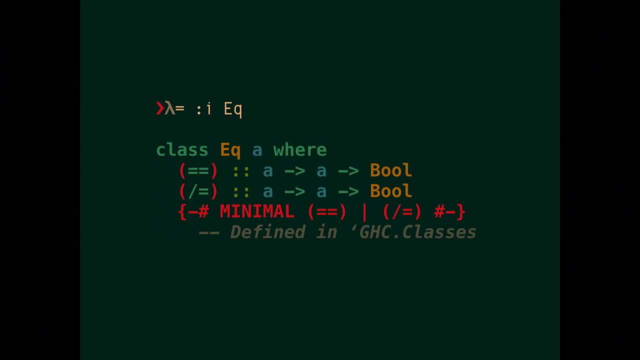 So we can ask Haskell for more information about the interface provided by a type class. In GHCI we can say colon I, which is info, So we can ask Haskell for more information about the interface provided by a type class, And that will give us the definition of equality. 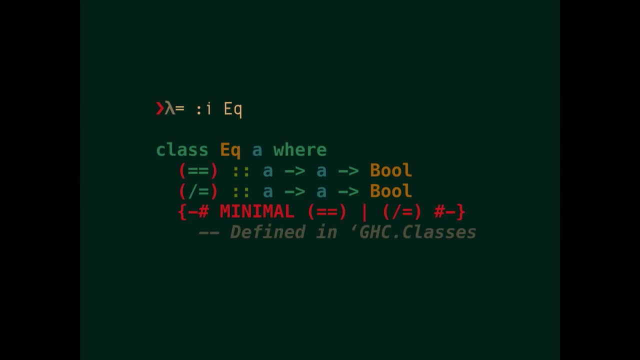 And we can ask Haskell for more information about the interface provided by a type class. It will also list all the types that it knows about that implement that type class And for eek. that's actually really long and so I've left that out. 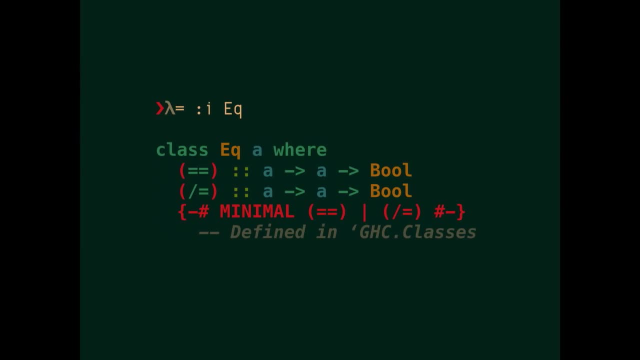 And yeah, colon I is a really useful thing to know. You can ask GHCI about types and type classes and whatever. So, yeah, the definition of the equals class or the eek class is that A is of class eek, where it's really a reference to examples. 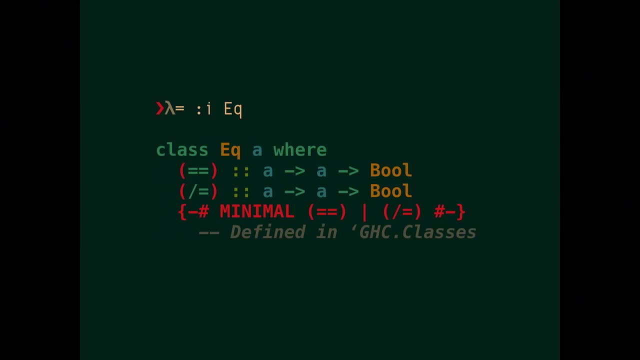 So you can ask. you can give us the number of times it's been given to you in terms of the size number, But the more than one time- in January of 2020, we'll be able to ask it for, because we вe got questions about how long it's been there. So we can say that we can ask that to GHCI. that's why we've been there And we can ask the number of times it's been given to you, which is eek. we can ask the name of the type, class, and that's EOO. 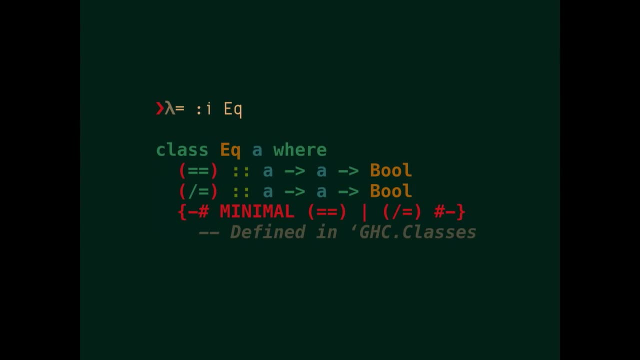 And the number of times it's been given to us, and that's ghci. So this is pretty helpful, And the other thing that we can also do is we can ask again for more information about the type class, So we can ask the same questions that we got from the G HCI class. 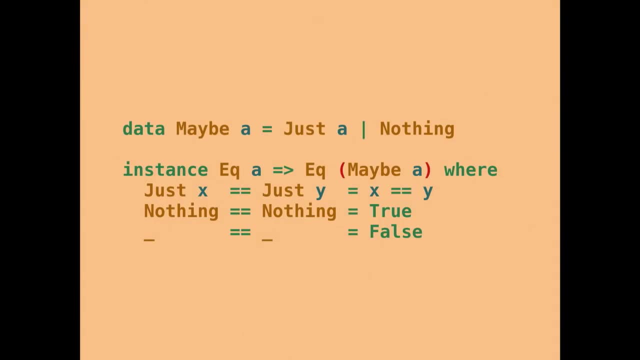 So, to give an instance, for instance, we can write our own instances for our own data types, or we can in fact write instances for other people's data types. So here's a simple data type called maybe. Maybe is sort of like a one element list. It could be empty it. 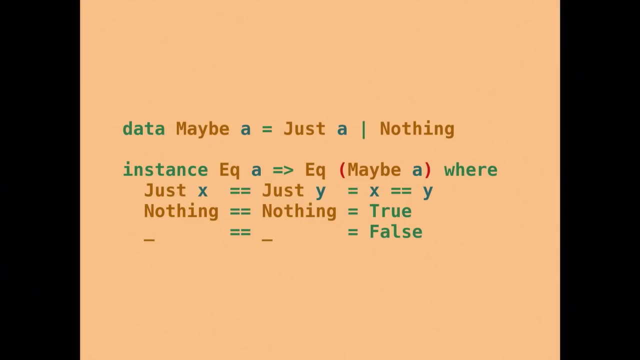 could be nothing or it could be just an A. So maybe A could be either just an A or it could be nothing, And an instance for equality. so now I'm telling Haskell how to compare two maybes for equality. So I say: well, given that I have an equality for A, I can build. 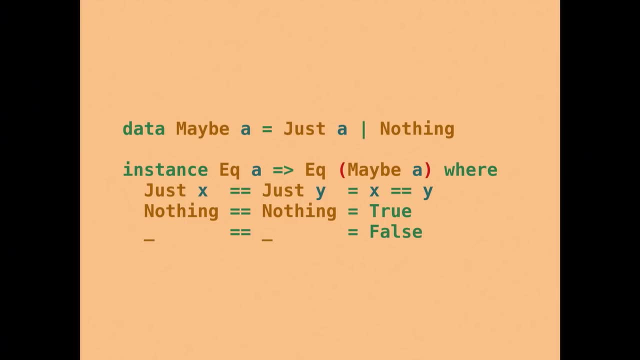 an equality for maybe A, where just X equals just Y, precisely when X is equal to Y And nothing equals nothing is always true and anything else is false. So we can define our own instances of these type classes, And in a lot of cases we don't actually have to. We can ask Haskell to just derive. 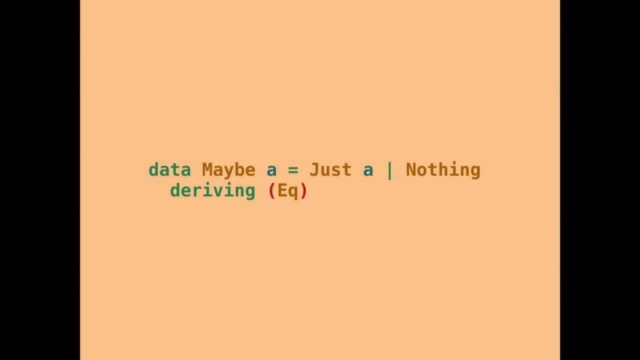 them for us. So, for instance, in the case of equality, we can just say this And this just says: do the obvious thing, which is what we just showed. Haskell has built-in rules to figure that out, so that's really awesome. Yeah, And the number classes that you can. 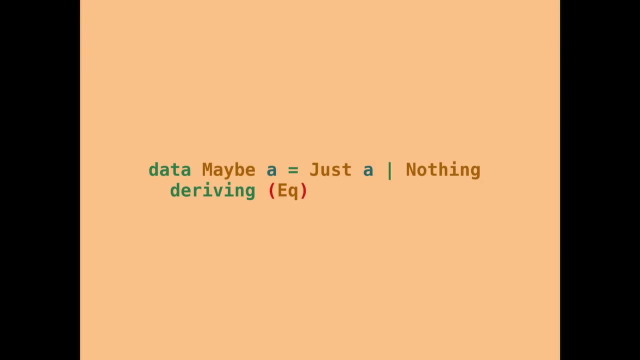 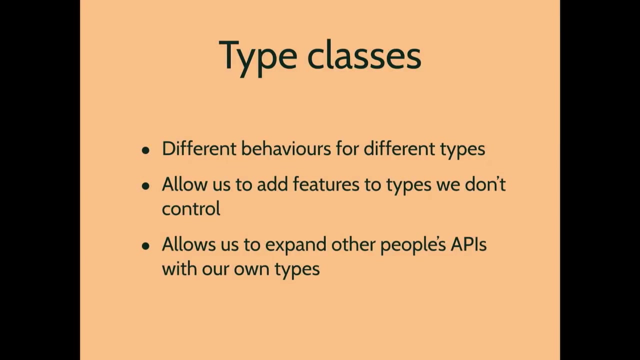 derive is constantly expanding, Mm-hmm. Normally it's like equality, ordering and some other things, but there are some pretty complex classes that you can now derive automatically in Haskell. Why do we care about type classes? Type classes give us this extensible coupling of behaviors with types, but at the same time, 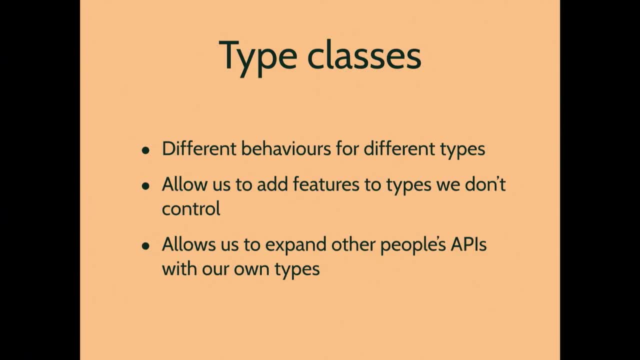 it decouples the type definition from the behavior definition. They don't have to be defined in the same place. We can have different behaviors for different types, and type classes allow us to add behaviors to types that we don't control. It's like adding methods to classes. 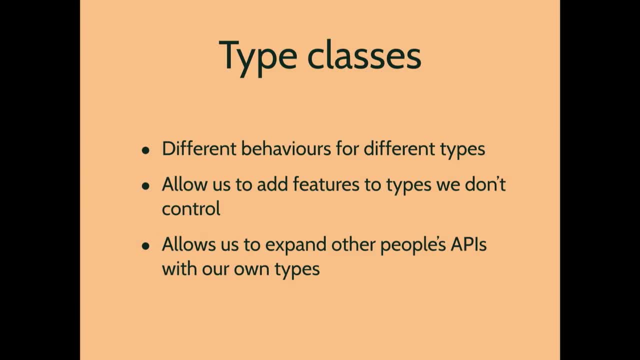 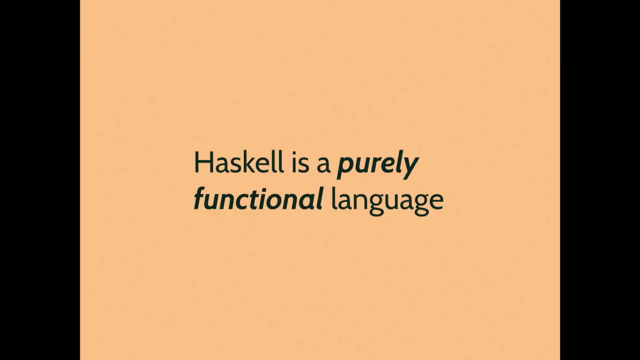 If you think in OO terms, it's like adding methods to classes you don't control. It also allows us to expand other people's APIs to use our types, which is super powerful. Haskell is a purely functional language and I promised I would say what that means. 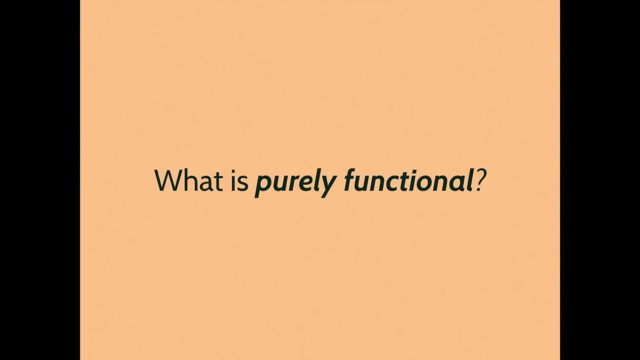 What does it mean? What is purely functional? Functional programming, I want to say, is not about first class functions, It's not fundamentally about functions being values. It's not about higher order functions like map or filter or things like that. 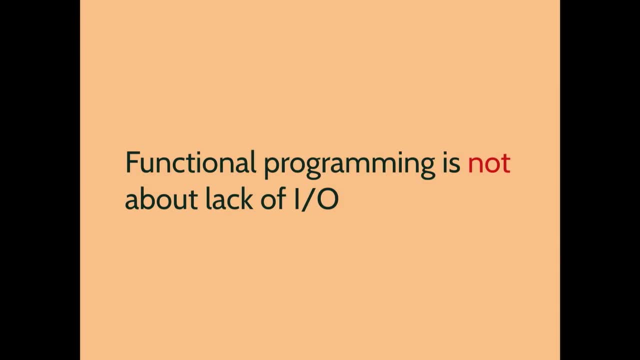 Haskell Functional programming is definitely not about lack of IO or things like that, because Haskell can definitely do IO and Haskell is yet purely functional. It's also not about immutable data. fundamentally, Haskell can handle immutable data in a purely functional way. 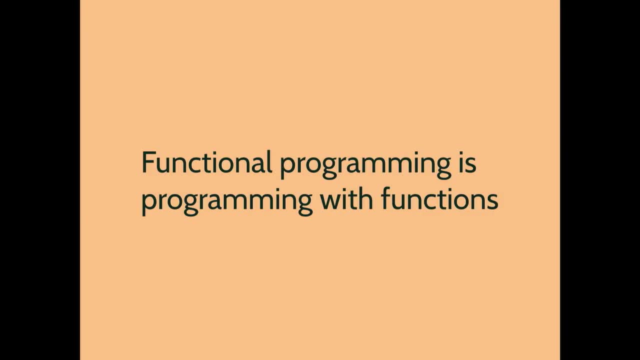 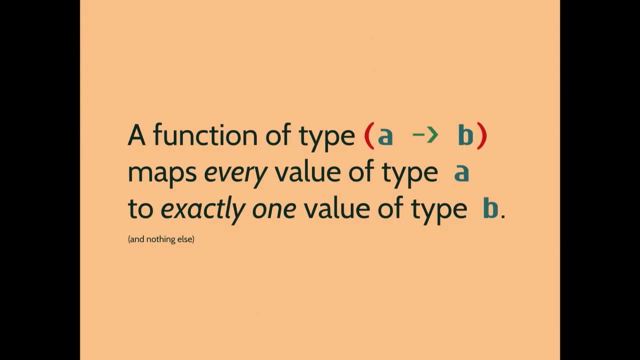 What functional programming is really? I want to say it's programming with functions. Functions in a very restricted sense, in the mathematical sense In Haskell. a function that has this type A to B. it has to map every value of type A to exactly one value of type B. It has to do nothing other than this. 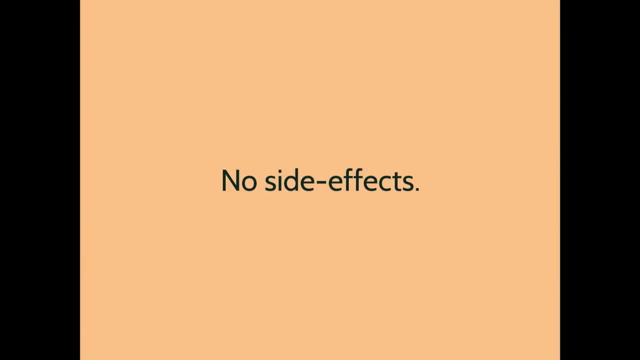 It just takes an A and it will give you a B and there's nothing else that happens. There are no side effects. Traditionally, when people think about side effects, they think about things like IO and mutating memory and reading files and they think, oh, you can't do any of these. 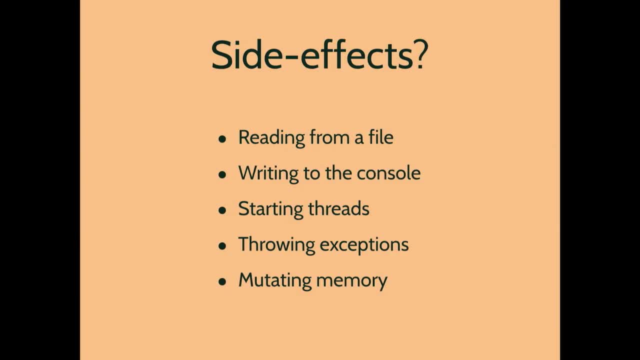 things. if you want to be purely functional, because there are side effects, Purely functional programming can't possibly do anything useful. but that's not true. You can do all of these things using just functions. Okay, The problem really here is that just listing things like this is not a good definition. 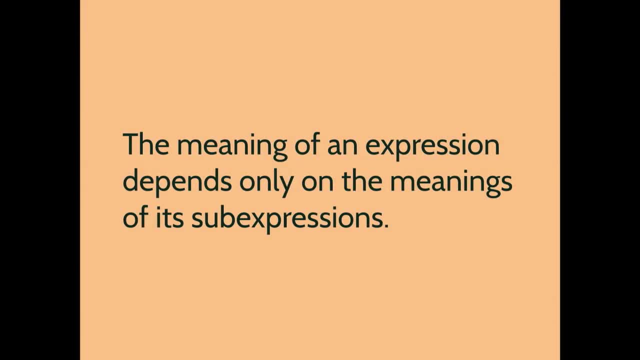 of side effect. A side effect is- I want to say anything that violates this property. That property is that the meaning of any given expression depends only on the meaning of its sub-expressions. When you see an expression in Haskell, what it means to run that program or evaluate that. 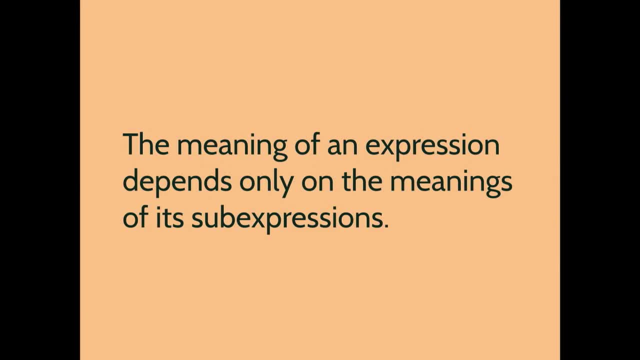 expression doesn't depend on any state outside the program. It doesn't depend on anything other than what that program actually means. It always means the same thing. A Haskell function will always return the same value given the same input. There are no external forces operating on a function other than its arguments. 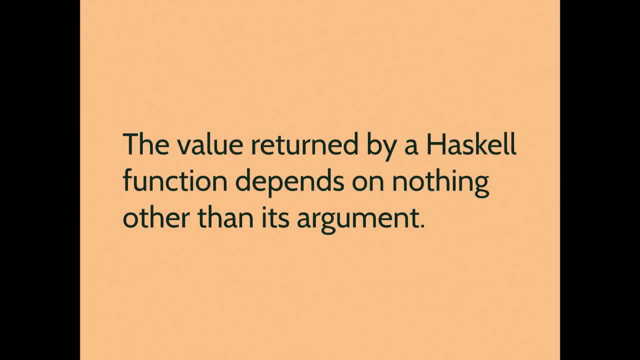 The value returned by a Haskell function doesn't have any hidden dependencies. There are no initialization steps that need to occur before you can call Haskell. It's always safe to call it, For example, for your tests. it's always safe to call Haskell function from your tests. 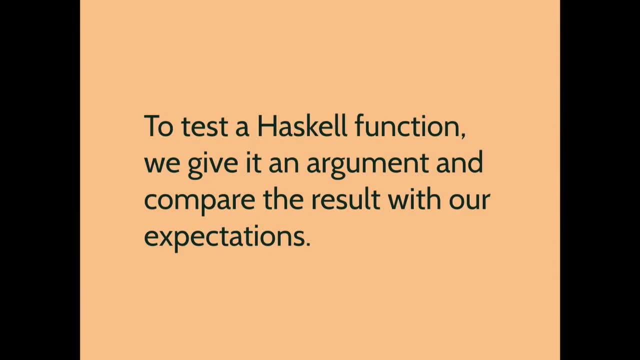 To test the Haskell function, you just call it and then you look at the result and you compare whether the result matches your expectations. When you're looking at the result of calling a Haskell function, you are looking at everything that the function did with your input. 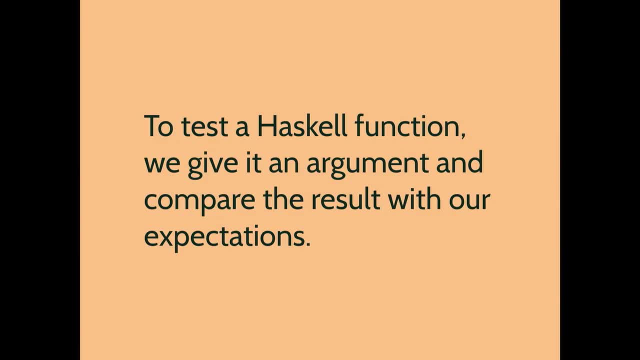 There's nothing else that the function could have done other than the return. You're just returning the value that you see. This enables this sort of computation model, where computation proceeds by simplification of expressions, just like solving algebraic equations. We can look at a simple example here. 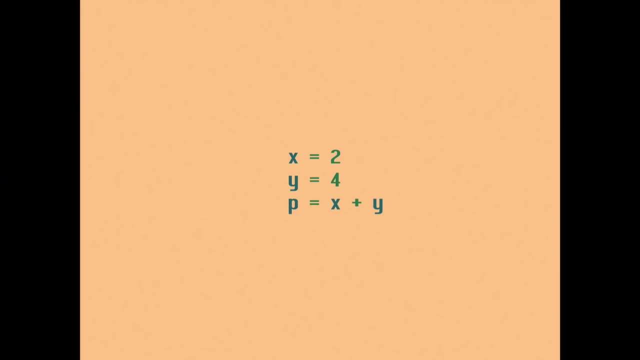 P is a program. It consists of some sub-expressions: x, y and plus. The meaning of P depends only on the meanings of x, y and plus. If we evaluate x and y and we can substitute them in to this expression, we get the same. 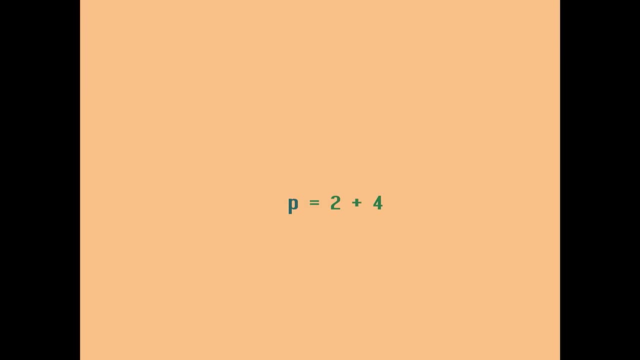 expression we started with. essentially It means the same thing. We can even go further. We can substitute in the meaning of plus as well. This P is the same as the P before. In Haskell Every program has this property. There are no Haskell programs that don't have this property properly. 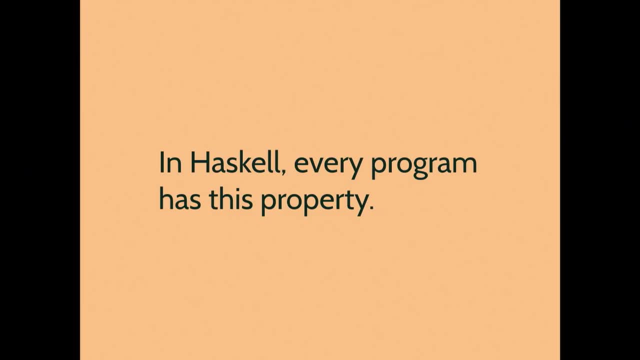 There are ways you can cheat, but I'm not going to tell you what they are. A Haskell program actually is a single, referentially transparent expression. I think that's sort of a cool thing. I'm going to show you a little Haskell program. 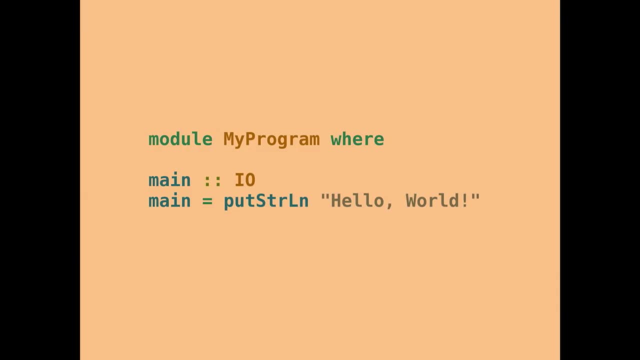 This is a little Hello World, Hello World. This program will print a string to the console. It prints out the string Hello World to standard out when you run it. If you look at what is the type of main, actually this is wrong. it should be IO with two parentheses. 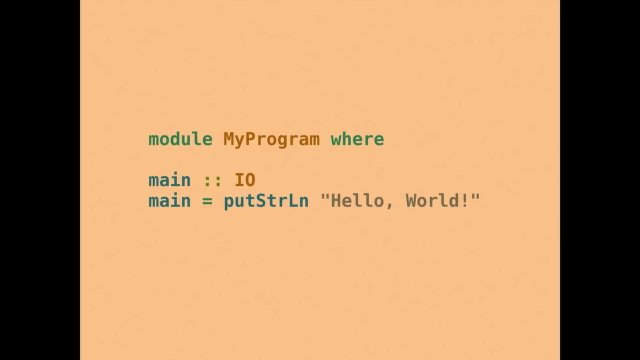 like that: It returns a value. This is a function Or an expression. The type of this expression is IO. What does that mean? It means that when the run time calls this function, it will get a value back. That value describes what the run time should do. 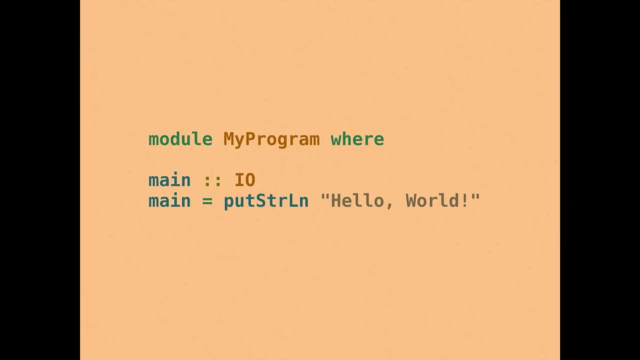 What the run time should do is print Hello World to the console. All right, Haskell, Haskell, Haskell. Although the Haskell Program doesn't do this, as a side effect, it returns a description of what should happen when the run time calls the program. 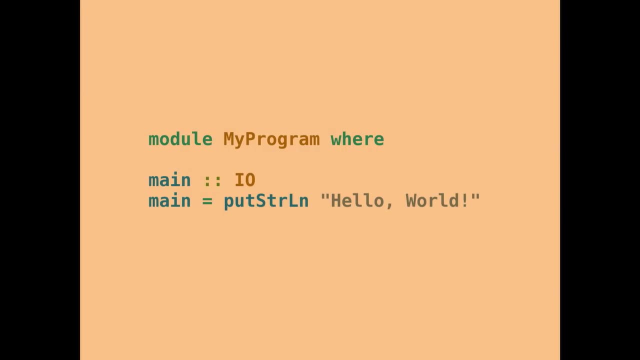 OK, So the only thing that can actually do IO is the run time system, So we cannot do IO in our programs. So then, uh, yeah, so what's the type of put string line that puts a string line to the console? 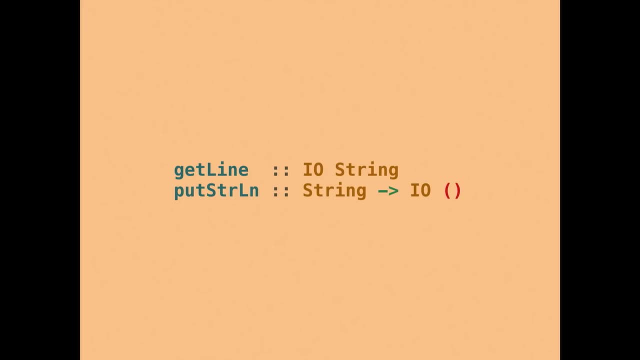 Uh, it's of type string 1. Other string that puts string to the console. type string to IO unit means it takes a string and returns one of these IO values. The open- close parenthesis means it has type unit or it's empty. It's a type that has no structure. 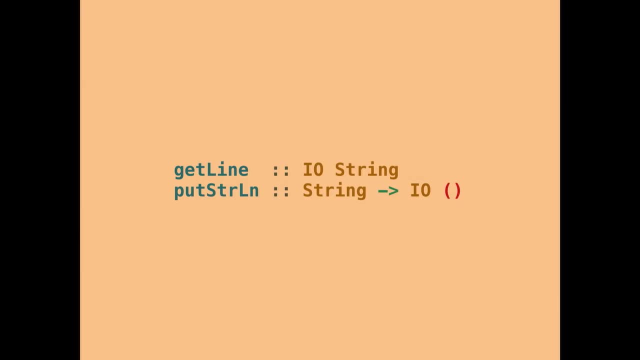 Get line is not a string, it's an IO string. It doesn't give you a string, it gives you an IO program that returns a string when it's passed to the runtime system. Then how do we put these things together? If we want to write a program that reads a 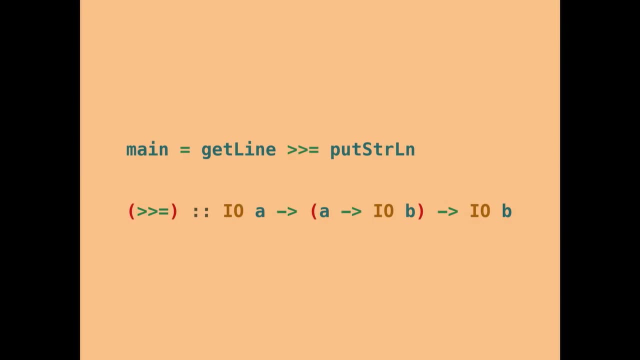 line and then prints it again. how do we put them together? Haskell has functions to combine IO programs as first class citizens To combine get line and put string line here. this is a program that will read a single line from the console and then echo that line back out. 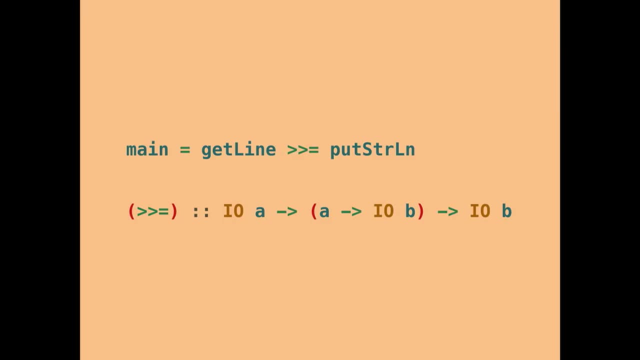 This operator here is pronounced bind. Bind has this type that it takes an IO of. A get line is IO string and it will take a function from A to IO. B put string line has type string to IO unit and then it will. 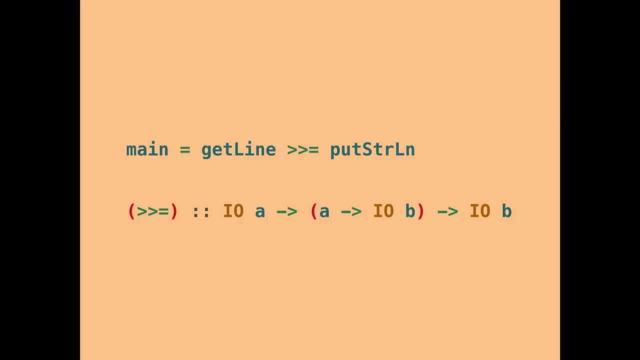 turn an IO of B, in this case an IO of unit, which is the correct type for main. This main will be a little IO script like this, that is a combination of get line and put string line. Haskell allows us to talk about IO operating. 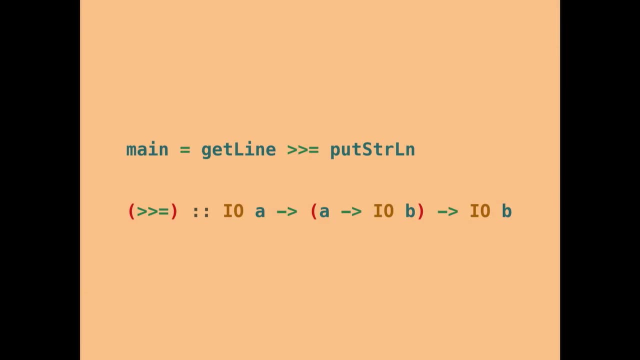 actions or programs as a first class citizen in the language, We can write the same exact program using what's called a do notation. When I say same exact program, this actually is the same program. It's just the syntactic. sugar for the bind. 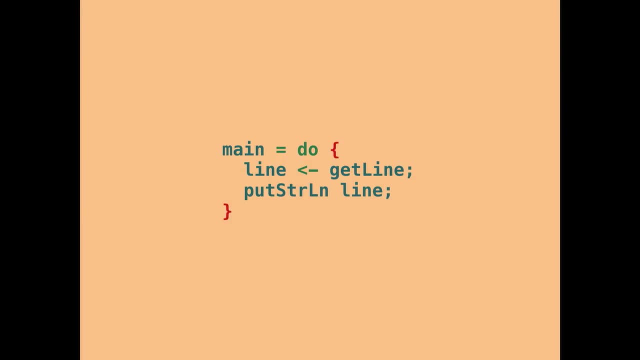 operator. Main here is the exact same program as main here In the syntactic sugar. we can write this as an imperative program. We say do and we can even put curly braces and semi-colons and it looks like an imperative. 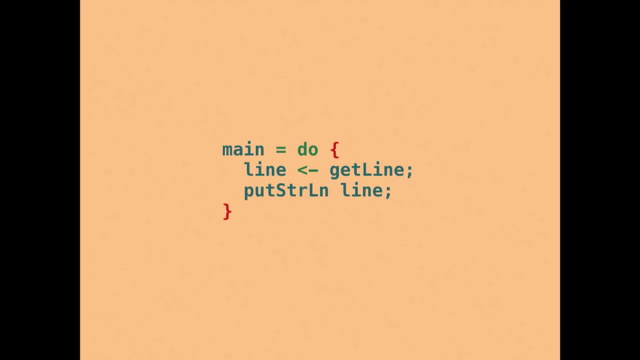 programming language. We say line comes from get line and then we say put string line of line. We can actually omit the curly braces and the semi-colons. in case you were worried about that, Haskell actually has significant white space. All you have to do is indent. 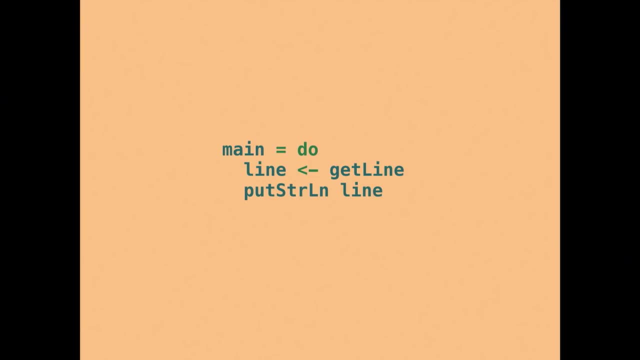 the block and you can omit the curly braces. The semi-colons are not necessarily, unless you want to put the statements on the same lines. Yeah, Haskell is actually a pretty great imperative programming language, because being able to talk about imperatives as first class objects in the language is pretty powerful, In fact. 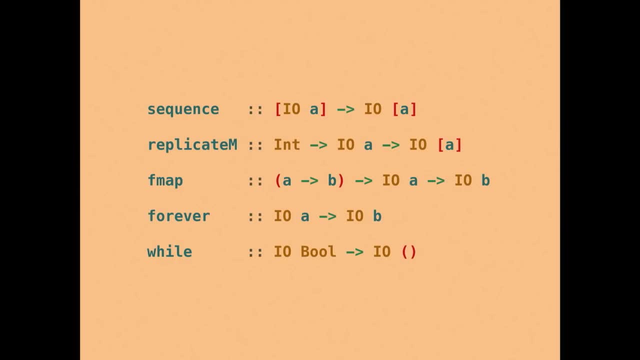 Haskell comes with a number of combinators or functions that operate on IO values like this. Just to highlight the top one here In the sequence: it takes a list of IO actions and returns an IO action of a list. The list will be all of the things that those IO actions returned. Here at the bottom while is actually 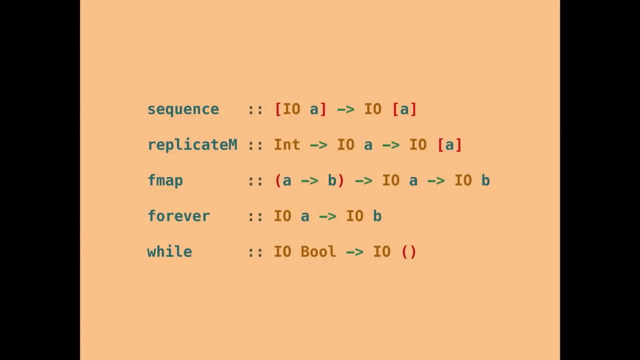 just a function. It takes an IO of Boolean and it will keep doing it until it turns to false. Haskell actually has no looping constructs at all. Everything is done by recursion. Repetition is always accomplished Here. for example, to sum a list, I'm doing this by pattern matching on the list Sum. 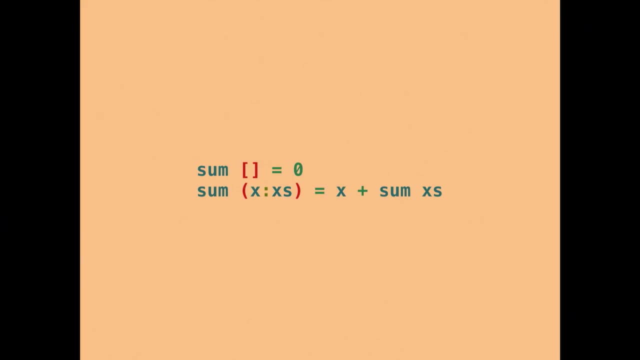 of the empty list is zero, Then I say sum of the list. Colon means construct the list. It's the same as cons, like a lisp Sum of the linked list with X at the head and Xs, as the rest of the list is just X plus the sum of Xs. It's a recursive definition. This is: 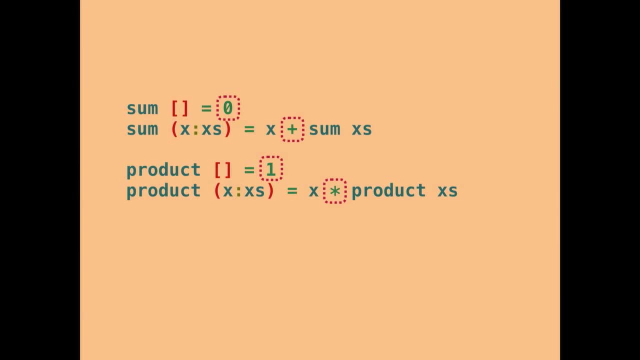 a pretty common pattern. We can write product in the exact same way experience, except it has one and times instead of zero and plus. These common patterns are often factored out into functions that we can reuse. In this case it's the function fold right. Sum is fold right with plus and zero Product. 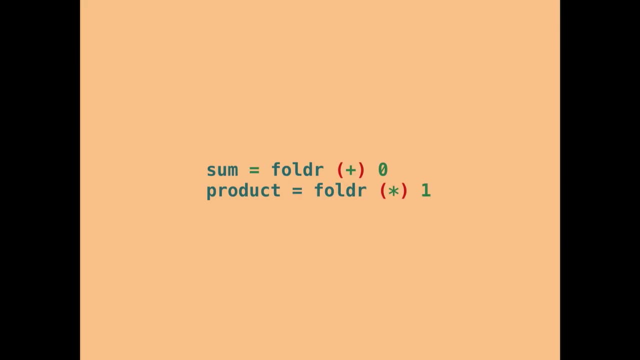 is fold right with times and one. There's also a form left which folds it in the opposite direction. Let's do this. I'm going to add: some went Okay, ready. We can reverse a list by folding it to the left with a flipped. constructor of the list. 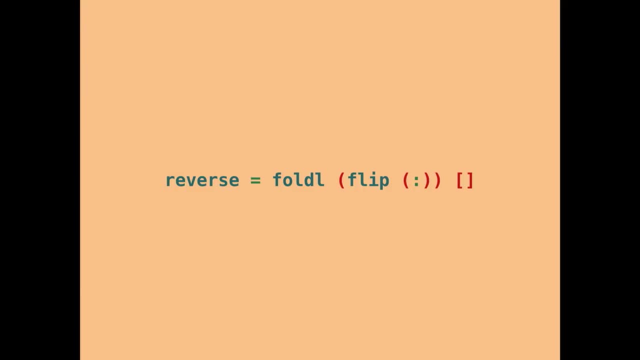 The next time somebody asks you to reverse a linked list on a whiteboard in an interview question, just throw this up at them: Fold left, flip cons, empty list- Great. Another cool thing about Haskell is that it isn't lazy. Laziness is something we're all familiar with from other languages, but Haskell is fully. 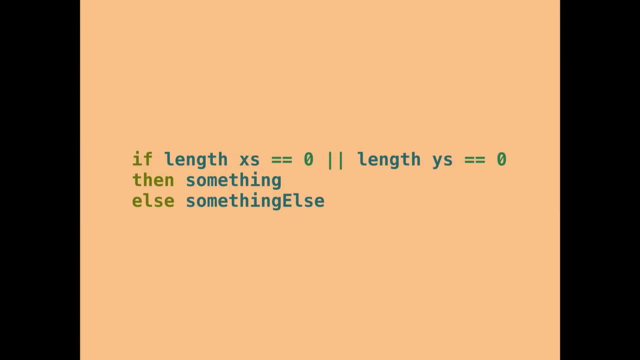 lazy In most languages. if we see something like this: if the length of x is zero or the length of y is zero, then something else, something else. We expect two things. We expect if the first condition here in this or is true, we don't even check the length. 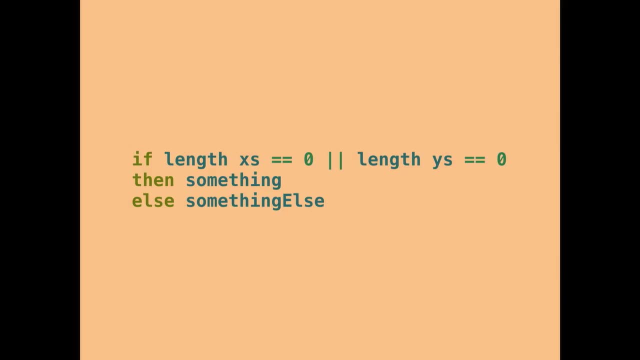 of y's. We expect this to short circuit. Also, we expect: if we execute the then branch, we don't even look at the else branch. We expect that to be lazy as well. In Haskell, everything has this property. Everything is lazy. 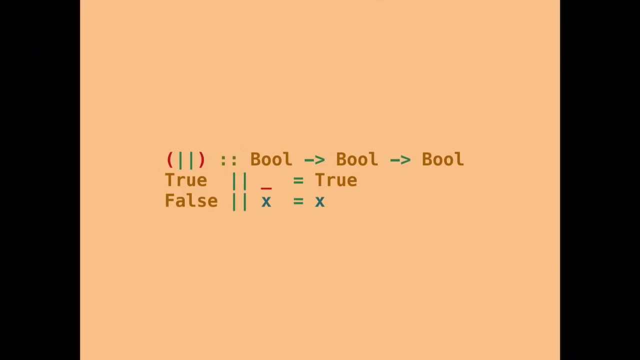 In fact or is not special. It's just implemented as an ordinary Haskell function. This says that true or anything is true and we don't even have to look at that other anything False or x is x. The magic here is that Haskell will not even look at x. 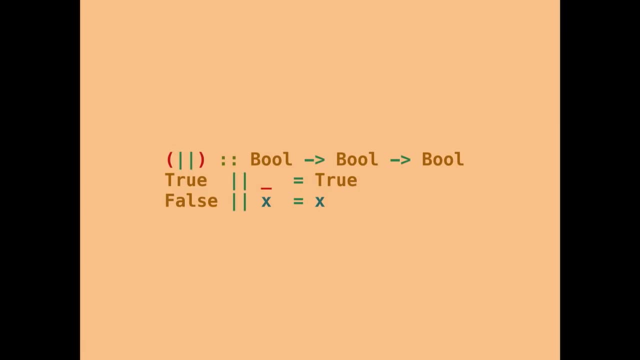 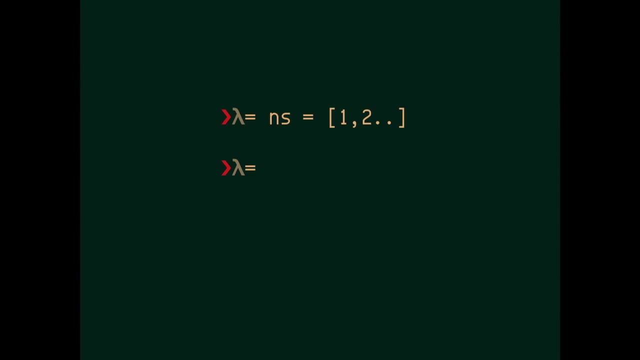 It will just return it, unevaluate it, All right. So laziness allows us to do cool things like construct infinite lists. I can say: well, n's is one, two et cetera. This is the infinite list of numbers starting from one. 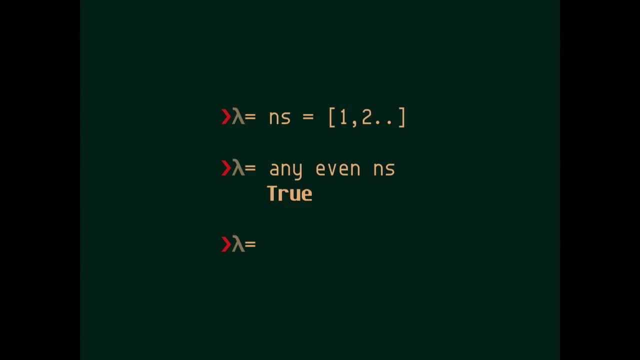 We can do cool things like ask if any of the elements of this infinite list are even. Haskell will come back and say, yeah, there are some even numbers in this infinite list. It doesn't construct the infinite list, obviously, but it will just construct exactly enough. 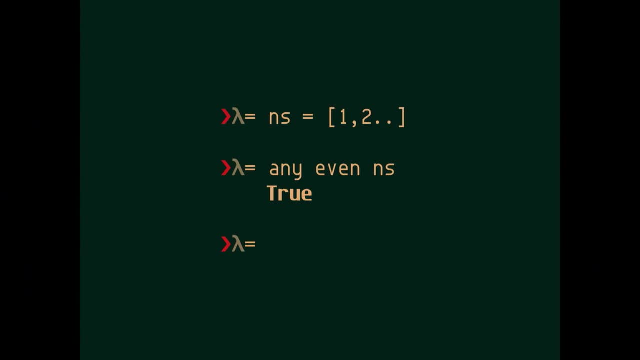 so that it can figure out whether any of them are even All. right. If you said all even, it would run forever. Or if you said are any of them less than zero, it would run forever as well. Oh right. 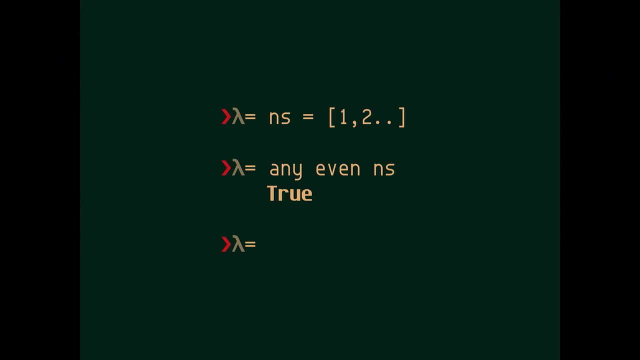 No, if you said all, even, it would also terminate, because the first one is odd. Yeah, you're right. Okay, Okay, Great, So any, and even here are not special, They're ordinary Haskell functions. This is not special syntax. 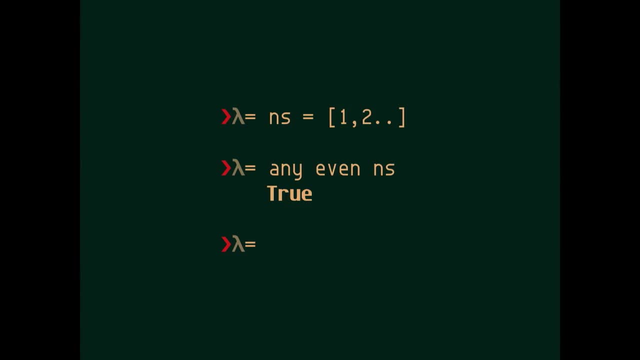 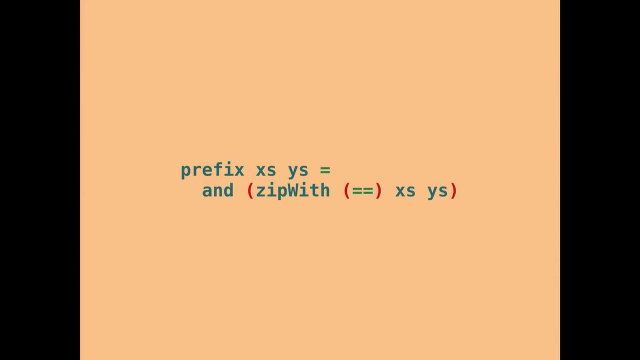 Any less than one would run forever. Yeah, Any less than one would run forever. Yeah, Any less than one would be an endless loop. Yeah, I think so Because it will have to look at the whole list to figure that out. 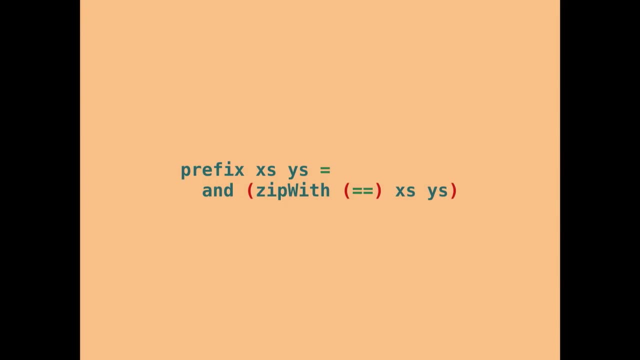 Okay, So this function here, prefix. it returns true whenever one of the arguments is a prefix of the other. So this zip with thing compares for equality of corresponding elements of X's and Y's, And prefix will return true if all of the comparisons are true. 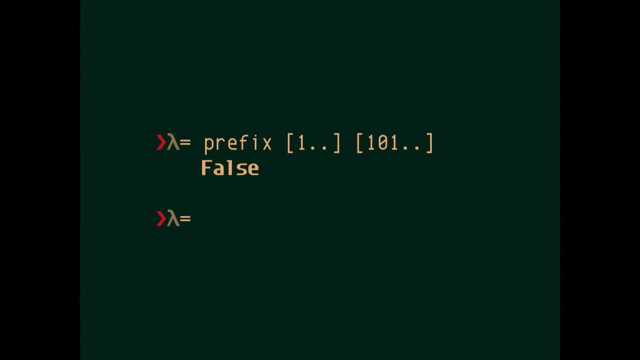 And we can actually do this with infinite lists. We can say, well, one et cetera is a prefix of one of the arguments. One et cetera is a prefix of one of the arguments, And then we can ask whether that's the case. 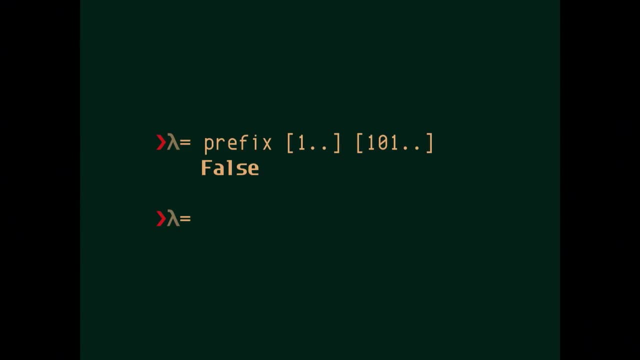 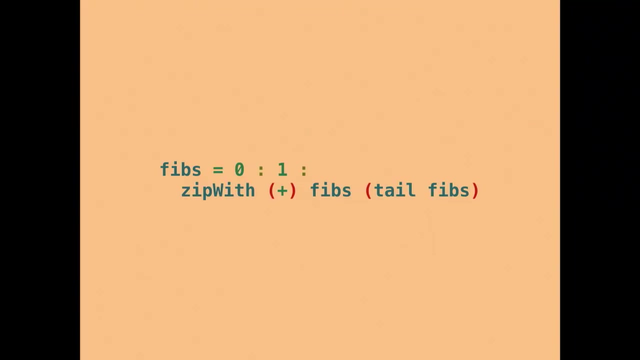 And then we can ask whether that's the case, And it will immediately say false, Because they're not equal on the first element, And so it immediately knows this must be false. We can generate the entire Fibonacci sequence as a list. It wouldn't be a functional programming talk if we didn't have Fibonacci's. 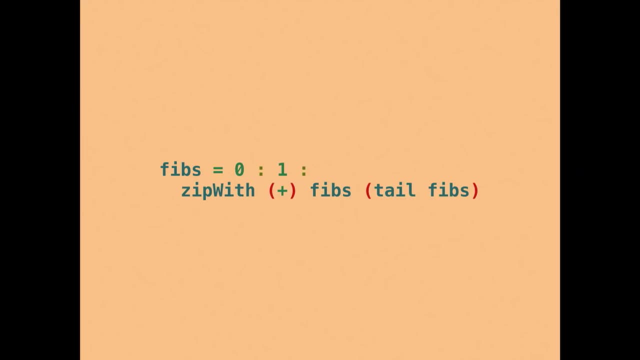 So we should say the Fibonacci sequence is zero, followed by one, followed by the element-wise or zip-width, the element-wise sum or plus of Fibs, FIBs, so the entire sequence, together with the tail of the entire sequence, So tail of FIBs, will start at one and then do zip width plus FIBs, tail FIBs. 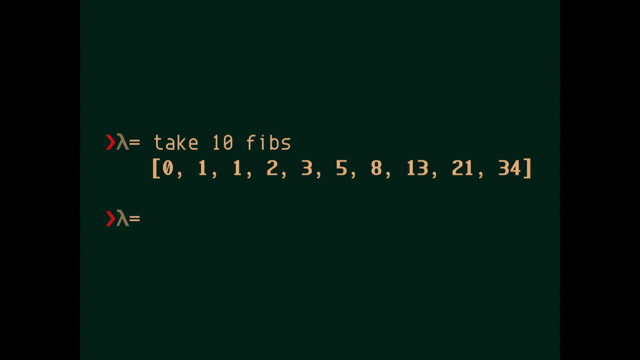 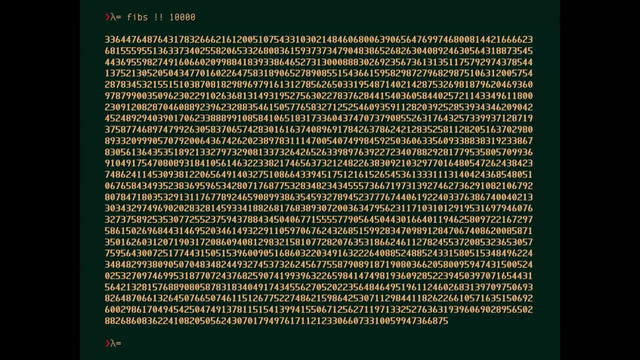 So this is the entire Fibonacci sequence, And then we can ask for the first ten FIBs, and it will give them to us, And we can ask for the 10,000th one, and Haskell will just say, yeah, that's fine. 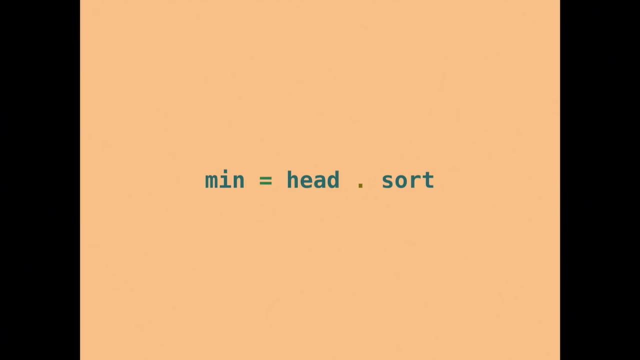 And in addition, this gives us this radical sort of code reuse. For example, if we want to get the smallest element of a list, we can just sort the list and then get the first element. Haskell will not only sort the list as far as it needs to. 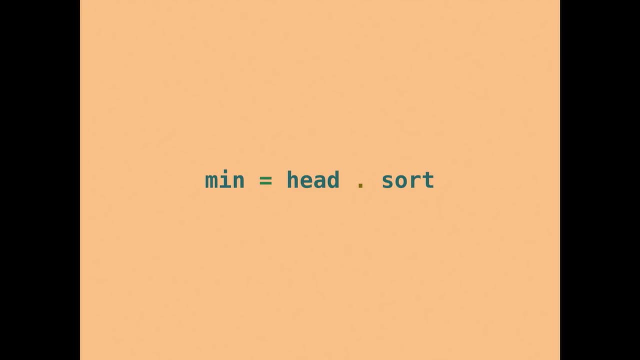 So it will actually only pass over the list once and it will find the smallest element. Because as soon as it finds the smallest element, it will put that at the head of the output list and head will be like: yeah, I got my. I got what I need. 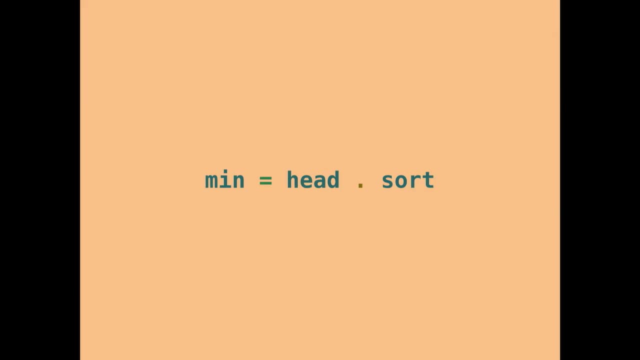 And so Haskell will allow us to do this sort of code reuse to write min in terms of sort In another language. This might be super inefficient because we'd have to like sort the whole list and then get the first element from the sorted list. 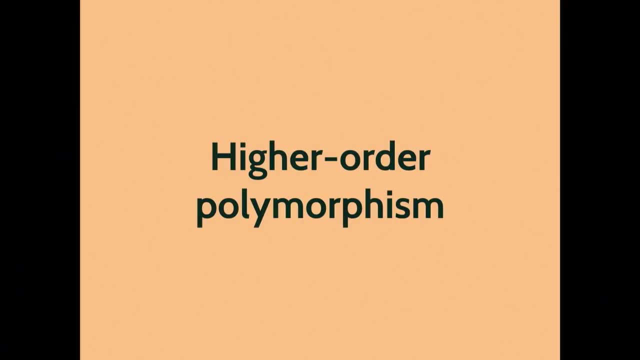 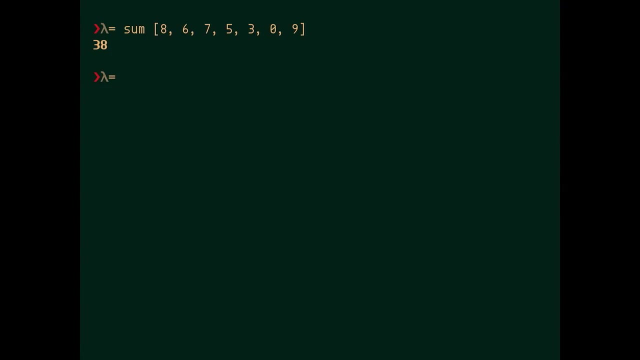 But Haskell will only do as much work as necessary. Yeah, the last super cool feature of Haskell that I want to show is higher order polymorphism, which is something that most languages just don't have. So if we sum a list like this, you know it's pretty straightforward. 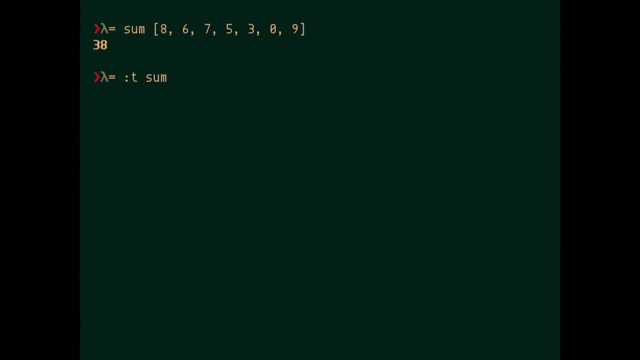 Operation. If we ask, well, what is the type of sum, it comes back and gives us this thing. It says: well, sum is of type T, of A to A, where T is foldable and A is a numeric type. So any T that you could fold, if it's full of numbers, you can sum all of those numbers. 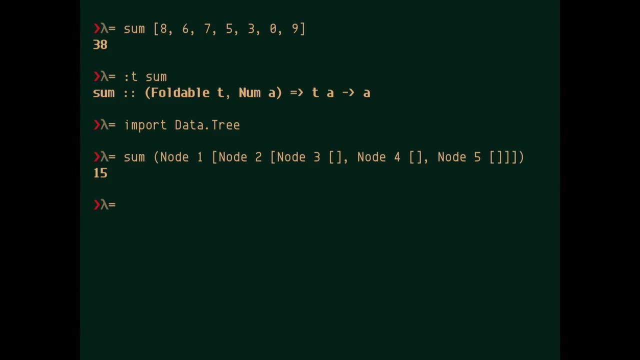 And list happens to be foldable. but there are other things that are foldable, like trees, So I can run the same function, sum. so this is not a different sum function, it's the exact same function. to sum a tree, yeah, Oh yeah. foldable essentially means you can turn it into a list. 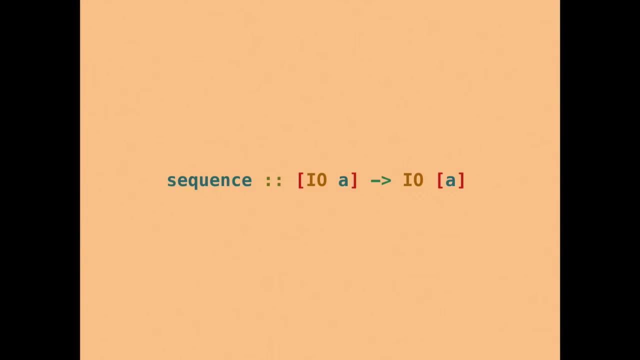 That's basically what it means. Yeah, Yeah, Yeah. So this would be like a. what is it called a pre-order or in-order? I forget which one it is, But it's like with a binary tree. it's like starting with the left most and going to the 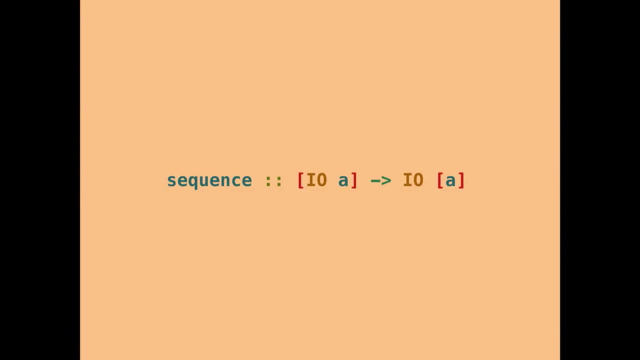 right most. So, if you recall this function from the IO portion sequence, which takes a list of IO actions and it turns that into a single action that returns a list of all of the results of those IO actions. If we ask what is the actual type of sequence? 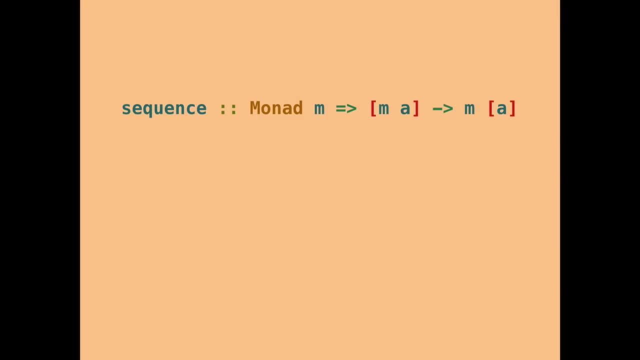 Haskell will tell us: well, the actual type is not specialized to IO. Real type says: well, as long as M is an instance of the monad class- Yeah, I mean, couldn't have Haskell without monads- As long as M has an instance of the monad class, we can turn the list of M's into an. 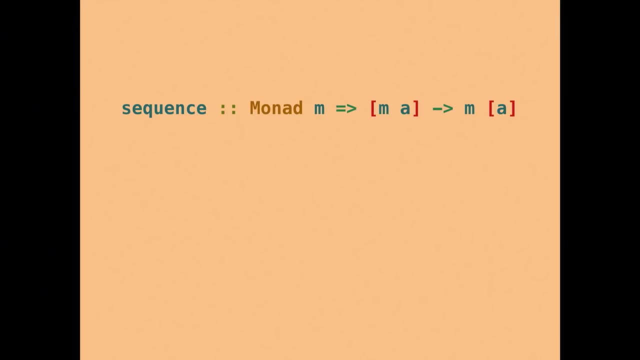 M of a list, right, And so M could be IO- right, But M could also be some other stuff. It could be, maybe. So sequence has all of these types. So sequence has all of these types, type for sequence. actually, it has a more general type than this, but this is as general. 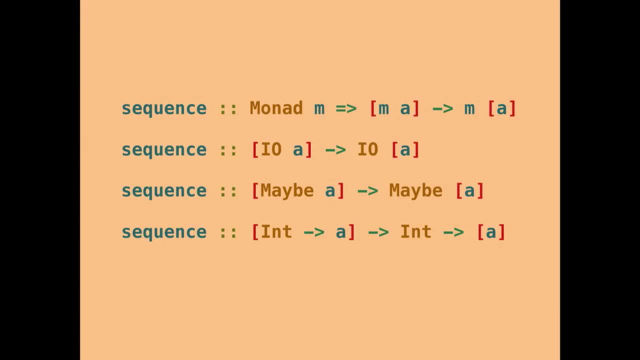 as I'm willing to go. The type of sequence is at the top, but it also has all these specialized types. If I specialize M to IO, it has that IO type, But it could also be maybe. M could be maybe, where I have a list full of maybes which might be. each of them could be an A. 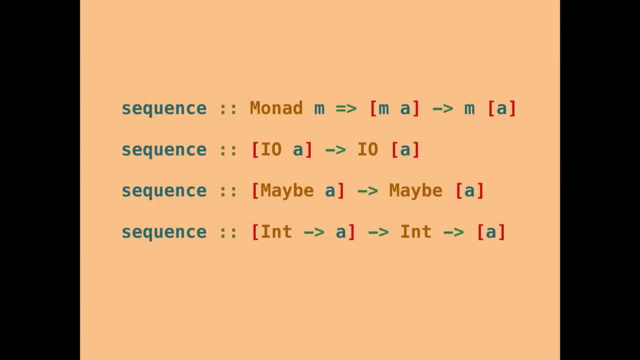 or nothing, and it will turn a maybe of a list and that maybe will be nothing if any of the elements of the input list are nothing. Otherwise, it will give me a list of all of the ones there, of everything, right. 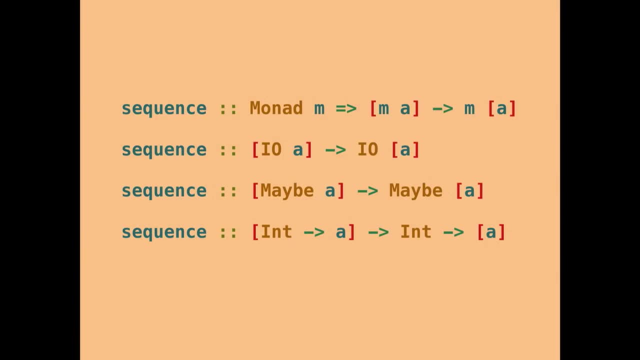 And functions also happen to be an instance of the monad class, and so I can take a list of functions that all take an integer and return an A, and I can apply them all to one integer And it will give me a list of all the results. right And crucially, this sequence function. 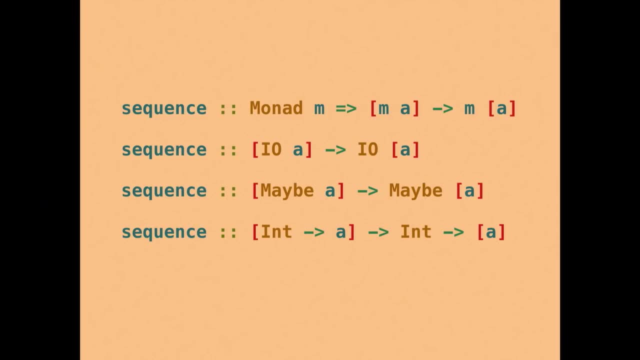 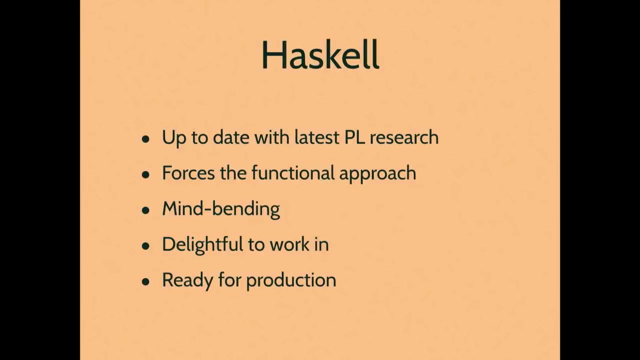 had to be written once for all of these types, and not just all of these types, but all future types that fit that monad pattern right. Totally awesome, Because lots and lots of things are monads. it turns out Right. so that's my sort of quick intro to the monad. 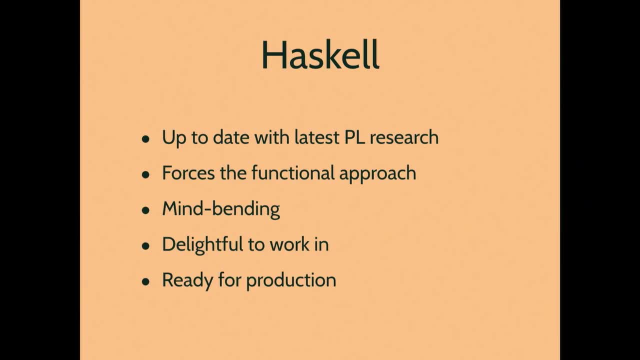 engine and I'm going to give you a little intro to cool things in Haskell. So Haskell, in summary, is very venerable, but it's totally up to date with the latest programming language research, and so if you don't want to wait 20 years for Java to implement some programming, 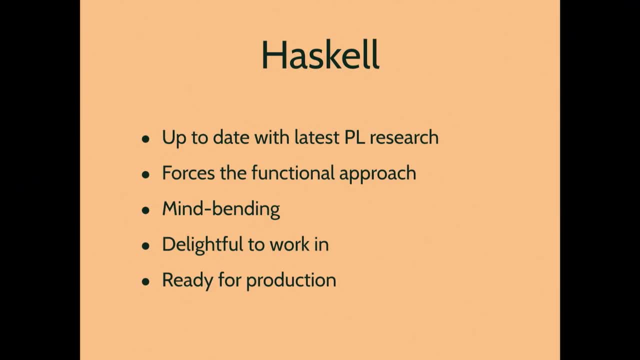 language feature. then just pick up Haskell and you'll probably have it. Haskell also forces the functional approach, so you can't fall off the rails. There are escape hatches, but they may as well not be there. Haskell is sort of mind-bending and I want to say: 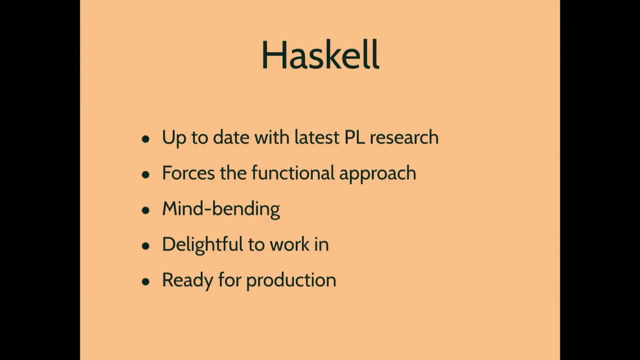 in a good way. It forces you to think differently about programming, and so if you want to sort of expand your mind about programming in general, Haskell is a good language to pick up, because it does force that functional approach. There's no cheating, And I actually just find Haskell. 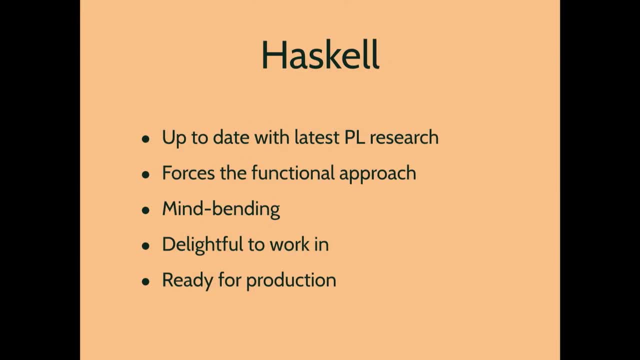 really delightful to work in. It gets sort of out of my way. It guides me through implementations using types. It's like my favorite language in the world. It's amazing. And also I want to say that Haskell is totally ready. It's not just like an academic language and it's not just something to do. 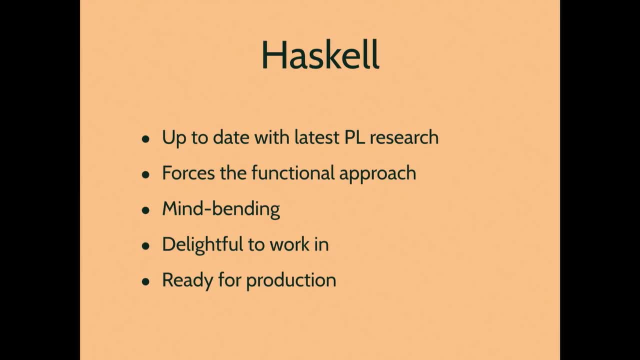 for fun. At TACT, we're using Haskell in production and it's super fast and amazing. It compiles to native code and we deploy it in Docker containers and it's servicing millions of customers and it's been really, really good. 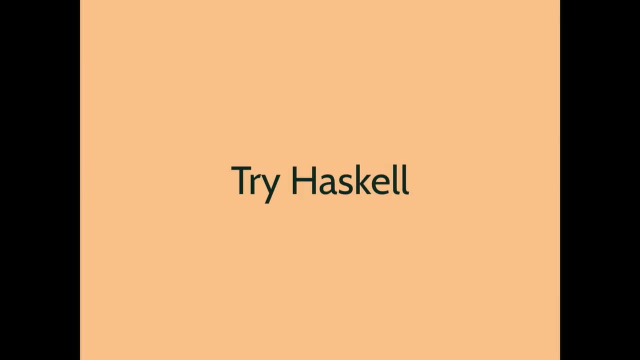 So I want to encourage you to try Haskell. That's all I got, Thank you. Do we have time for questions? do you think Five minutes for questions? Any questions about Haskell? Yeah Right, Well, let's go back to the read line. 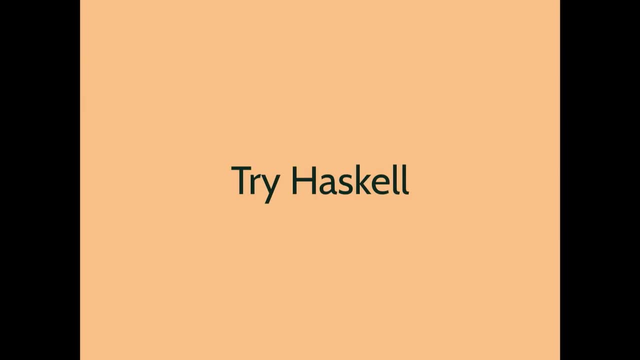 Well, let's do a simple thing like read line. right? So get line definitely has an effect, right? It doesn't have a side effect in the sense that the meaning of get line actually just depends on nothing other than that. But the 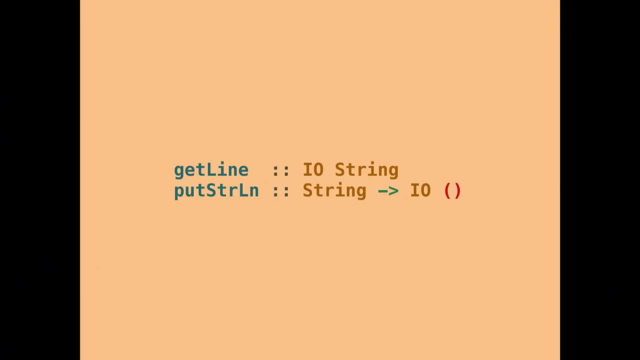 way it actually then produces. is one of these IO scripts, right? And the important thing is that you actually cannot look at that string, right? You say get line, you don't get a string. You can't take the length of that string, for instance. What you have to do is that. 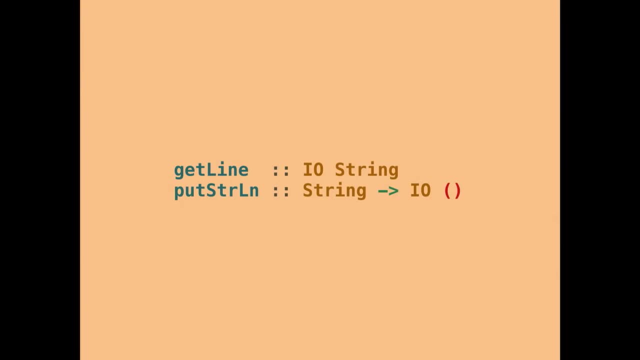 you have to return that IO string to the runtime system. But if you want to then inspect the string or put the string to the console, you also have to tell the runtime system what to do next once it has that string right. So all of the effects happen outside of your program and are therefore 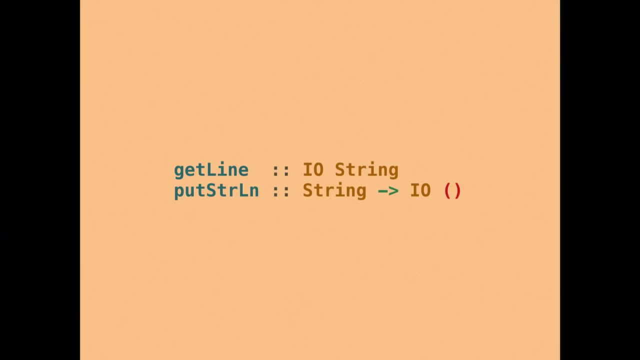 not side effects. Does that make sense? I don't know. Maybe a cool thing to think about here is like if you have asorry in Haskell, you could say get line, and you could put get line like four times in a list. 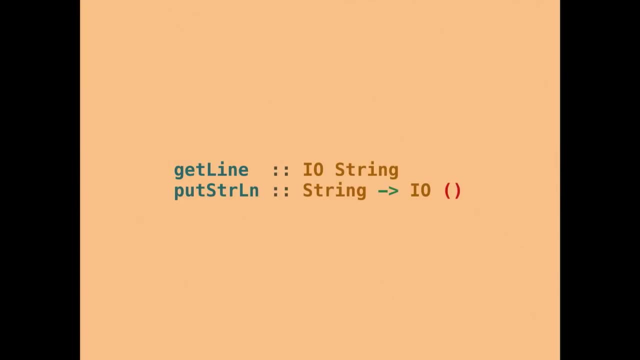 There's a list of four. get lines right, Then that sort of thing can go away. Special property: So if you wanted to do something like run virs and get vr and get all the things, and then we're not sure if that would make sense to use or not to use these paternal types. 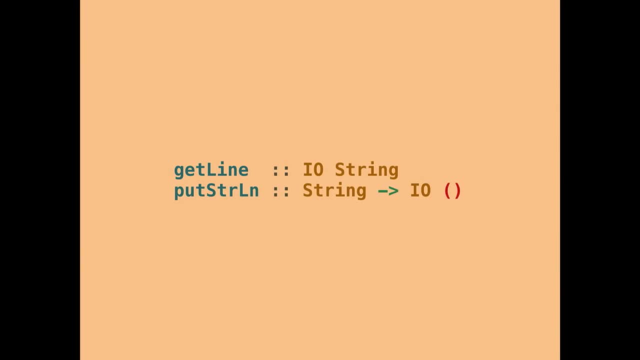 Not necessarily possible. Yeah, Yeah, Yeah, Yeah, Yeah, Yeah. So you won't be. when you look at that list, you won't be getting any lines. All you're getting are these I-O strings. Male Speaker 2 in audience. Okay, 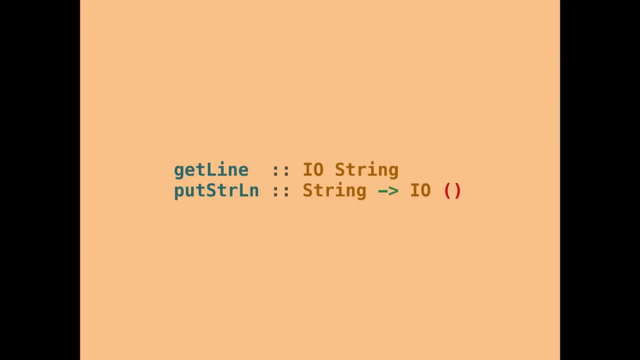 Male Speaker 2 in audience. Sure, Male Speaker 2 in audience. Oh, what is the strength of Haskell? I think the strength of Haskell is the purely functional programming, Like, basically, if you want to do purely functional-. Male Speaker 2 in audience. What's the strength of purely functional? 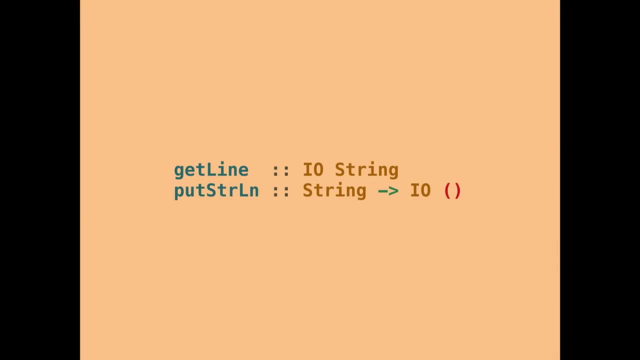 programming: Male Speaker 2 in audience. Oh, you mean in terms of a specific domain: Male Speaker 2 in audience. Yeah, I think actually all domains benefit from this approach, But I think the closer that your domain is like to- Male Speaker 2 in audience- mathematics- the more you're going to get. 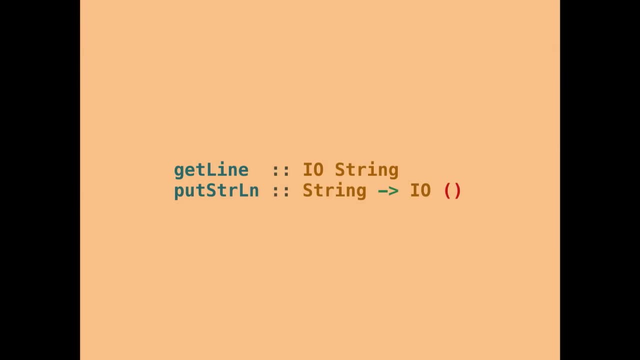 Like finance. Haskell is super popular in finance. It's very popular in other things like that. Yeah, that's our question. Male Speaker 2 in audience. You have to optimize for understandability, So it will come back to your code half a year later. 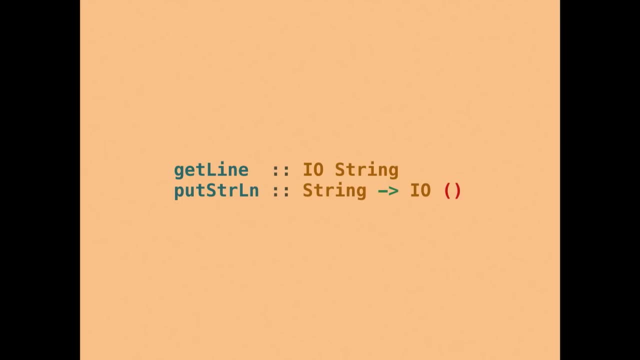 Because you have this purely functional approach that you can ensure that the function doesn't lie and it doesn't have side effects. you look at the definition of the function and you don't need to check the server that you're using. Male Speaker 2 in audience Right. 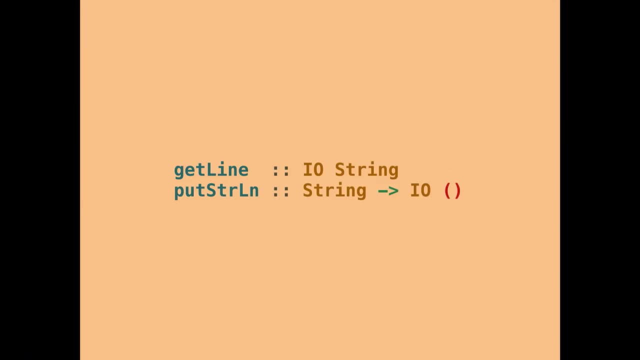 Male Speaker: 2 in audience. I guess the answer then is: the suitability for a domain is not like a yes or no thing, It's more like a scale, And I guess, to the extent that your program is like sort of throw away, the less you're. 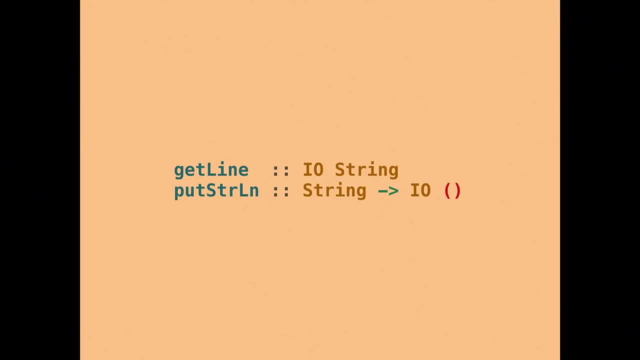 going to benefit from Haskell, The more you have to maintain your code base over time. Male Speaker 2 in audience. Yeah, Male Speaker 2 in audience. The more you have to sort of totally understand what your program does, the more you benefit from it. 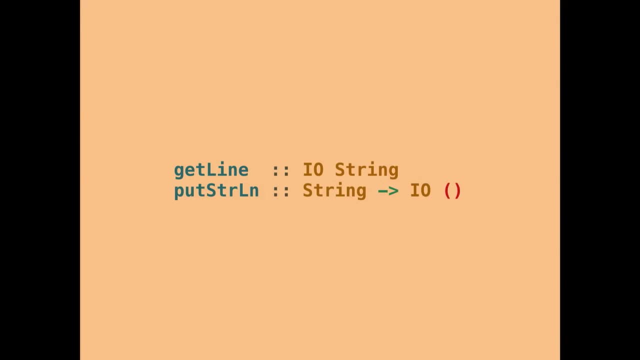 Like, if you're just throwing up a website that you want to show a client like as a quick thing, like Haskell might not be a good fit for that. Male Speaker 2 in audience. Yeah, The more complex your reasoning, the more applicable it's going to be. 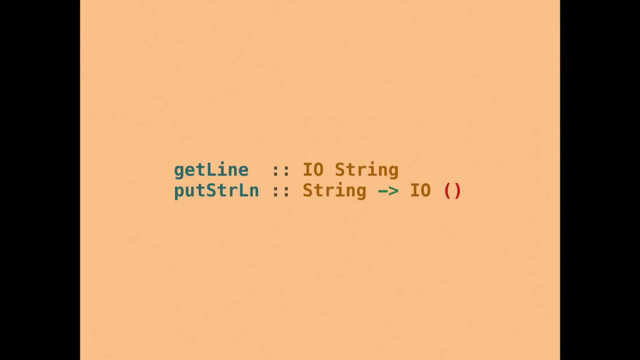 Yeah, definitely Male. Speaker 2 in audience: Pretty rich, I mean. Haskell has been around for a long time and so there are lots and lots of packages, Lots of awesome cool libraries that I didn't mention. Like Servant, for instance, is a web service framework where you can just like, specify. 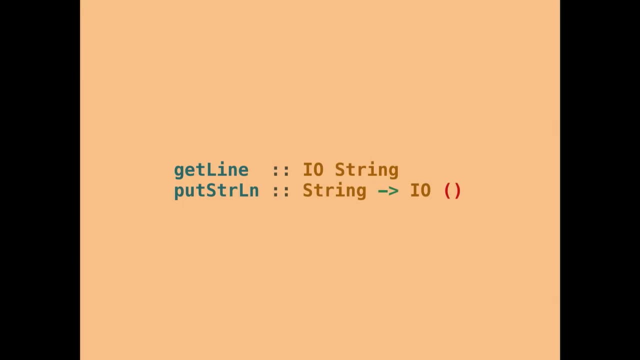 the type of your API and it will generate a web server for you that implements that type. It's like totally awesome. Male Speaker 2 in audience. What's that? Male Speaker 2 in audience. Yeah, Male Speaker 2 in audience. Oh, there's a package management system. 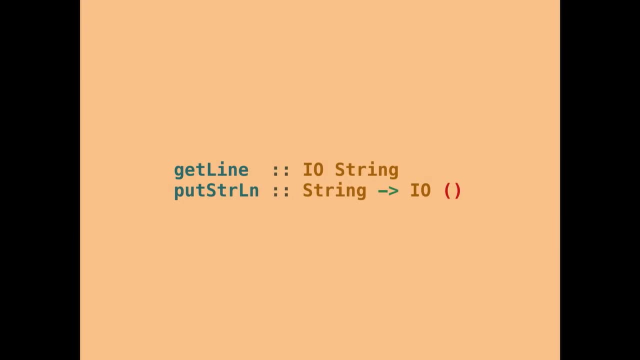 yeah, Cabal, and there's also Stack, so there's more than one package management system. Male Speaker 2 in audience, I think. so I think they can interact. but like, yeah, And there's Hackage and then there's Stackage, so yeah, 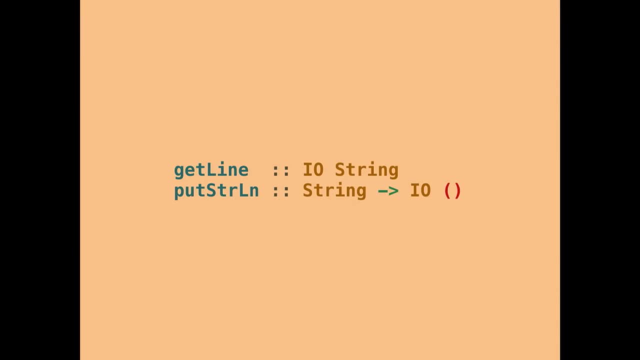 Male Speaker 2 in audience. They use the same packages but they use different implementations of the repo. Male Speaker 2 in audience. Doesn't it have a clever search engine that lets you search Male Speaker 2 in audience? Oh yeah, That's another thing. 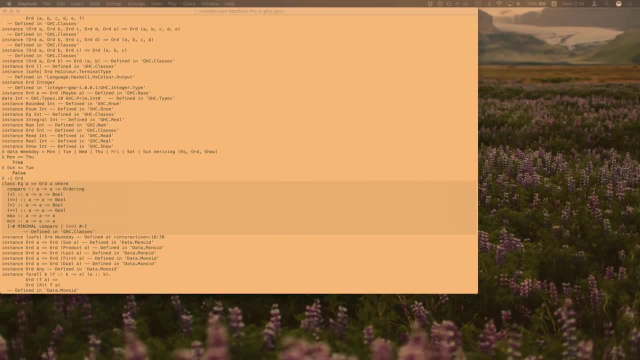 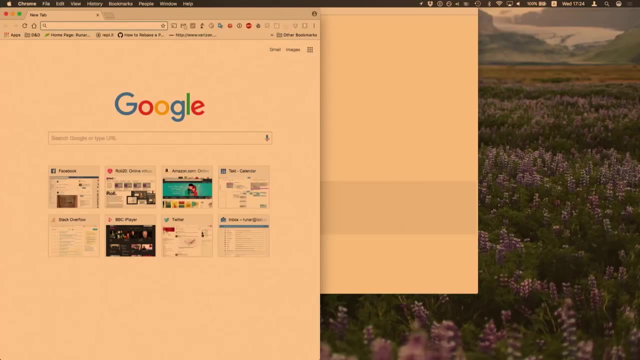 Like you can-. yeah, Maybe I can show that to you. Male Speaker 2 in audience. Who, yeah, Who go- or actually HeyU is better. Am I over time now? Probably Male Speaker 2 in audience. You should probably close up. 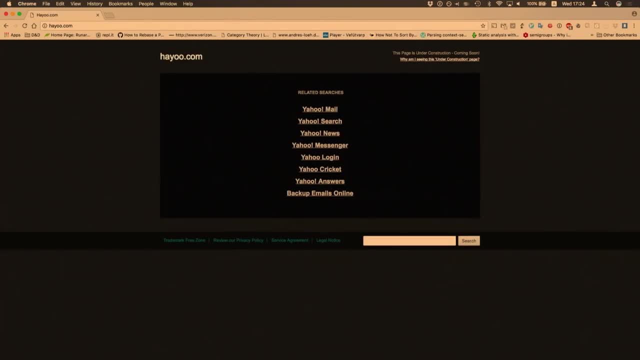 Male Speaker 2 in audience. I should close up. Male Speaker 2 in audience. Oh that- oh no, It auto-corrected to Yahoo. No, HeyU. Oh no, it's not actually heyucom. Oh no, I don't know how to get there. Go on. 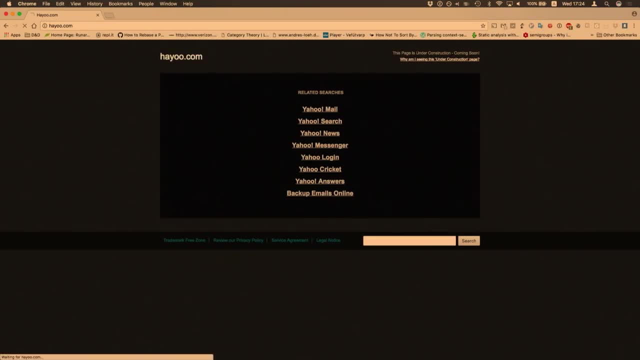 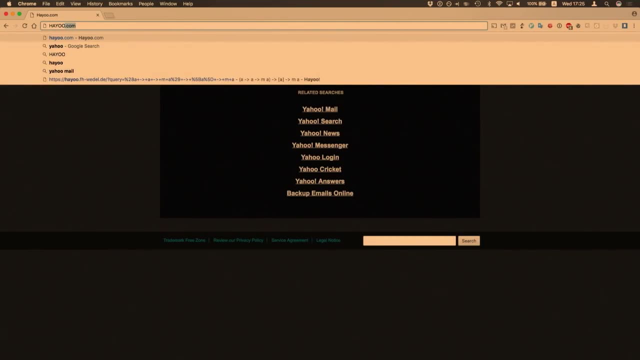 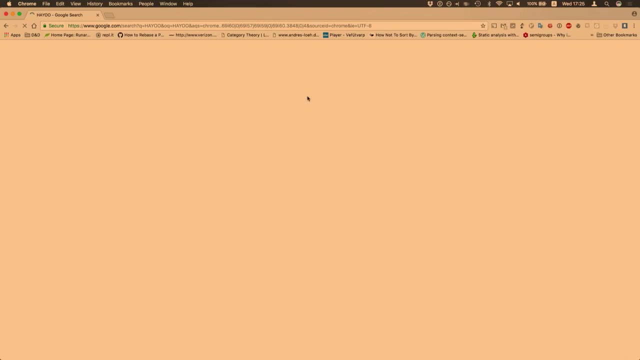 Oh, it's heyu. This is when I do a Google search for it. It's like you type in a type signature and it gives you a list of functions that implement that type signature in the libraries, in the Haskell libraries: heyu, Haskell API search. Let's say I want to find